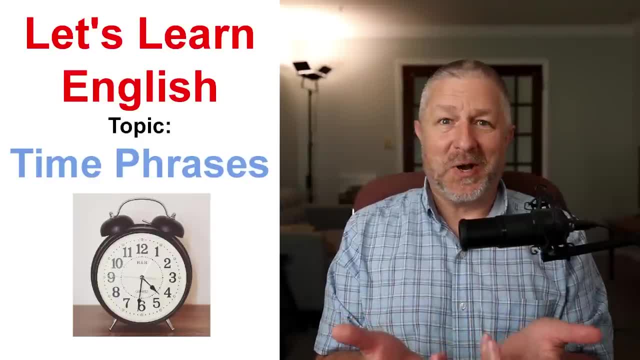 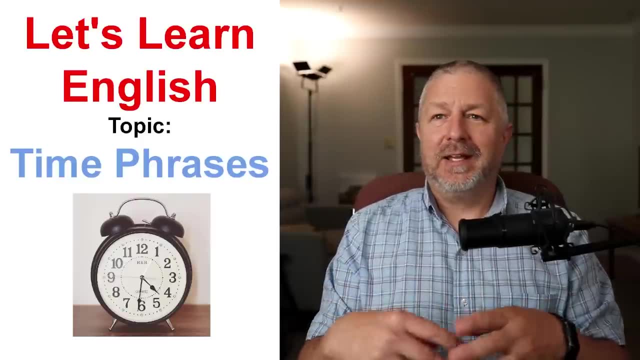 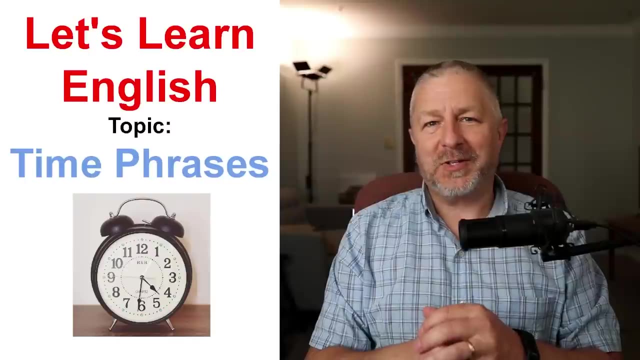 can talk about time better. As humans, we talk about time a lot. I had to get up at a certain time this morning and I had to do a few things before this lesson started, and there are a number of ways to describe how we view time and interact with time as human beings. So 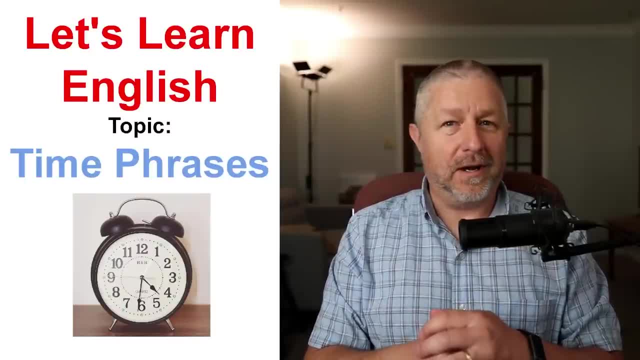 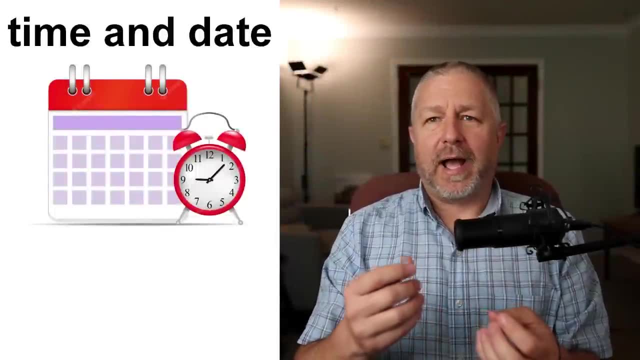 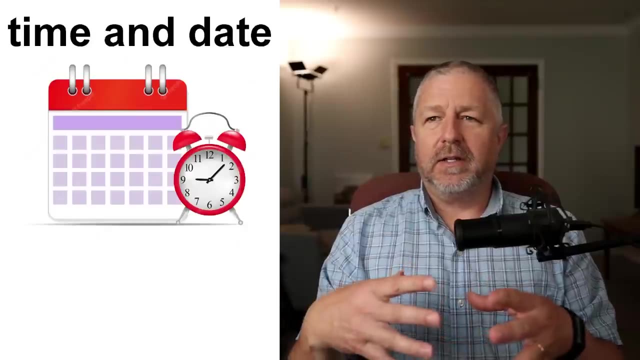 once again, welcome to this English lesson about time phrases, Time and date. So these two words often go together in English Whenever you have an appointment. So if you have a dentist appointment you have to remember the time and date, So they're not always together. I said: 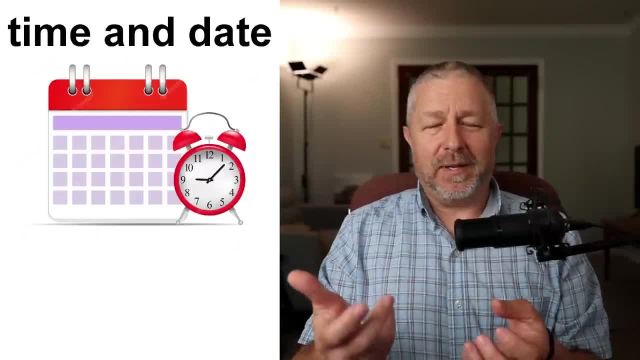 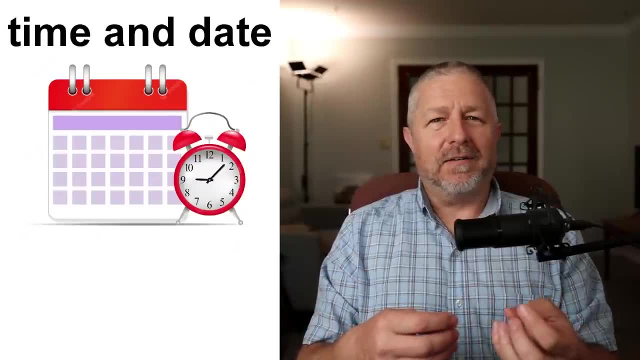 they're together quite often. but, yes, you need to remember the time and date. Um, you need to remember the time and date for a doctor's appointment. You need to remember the time and date of, perhaps, a movie you're going to go see. Maybe you're going to go see a movie with a. 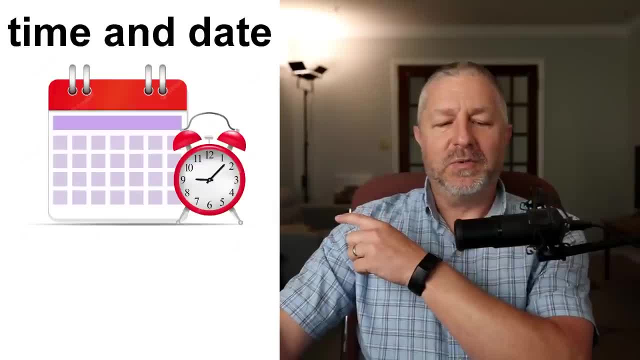 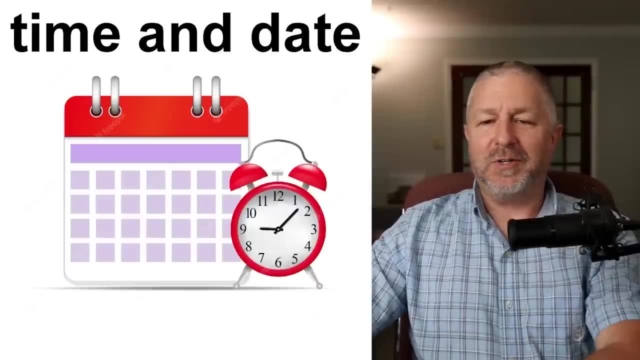 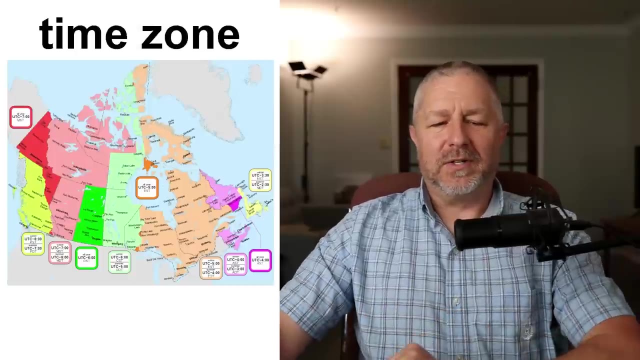 friend this coming Saturday, It would be very important to remember the time and date so that you can be on time. Uh, it's good to be on time for things, and you can be on time by remembering the time and date that something happens. Time zone, So a time zone is the place on earth where 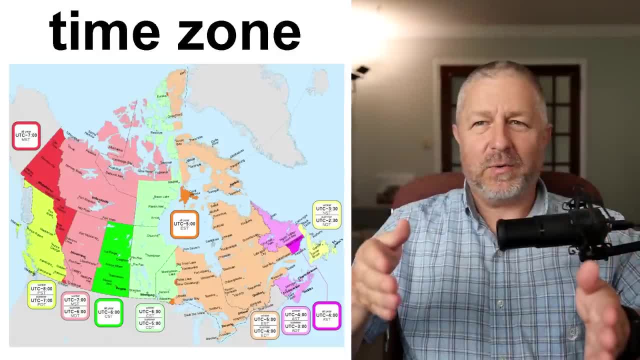 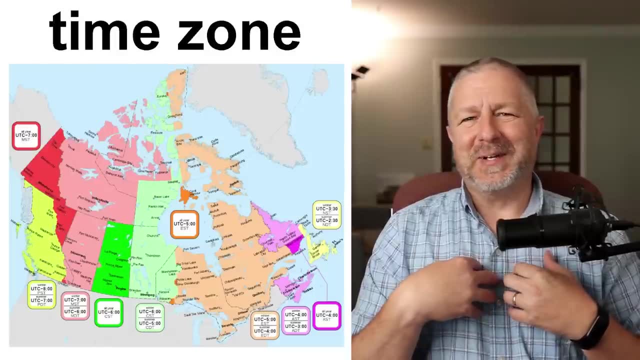 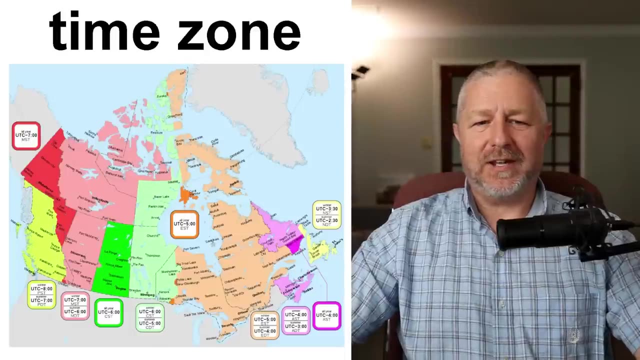 you live and the name of that zone based on time. I live in a time zone in. I live in Ontario and my time zone is I am in eastern standard daylight savings time. We usually just say eastern standard time, but right now it is 834. 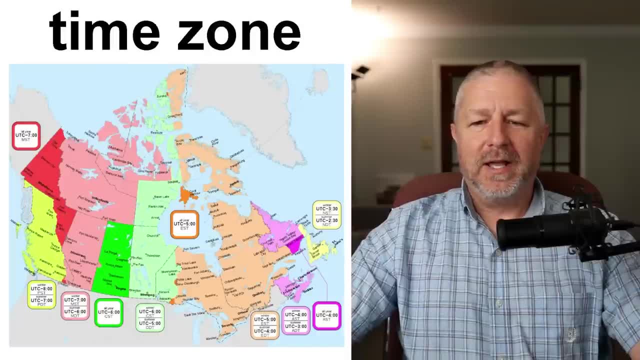 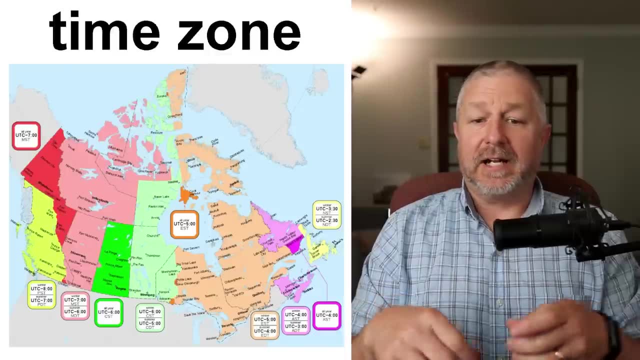 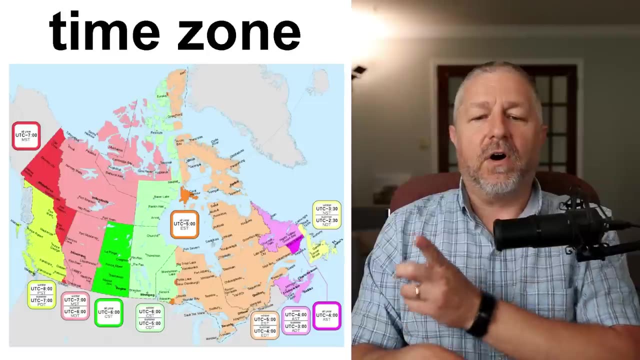 AM where I am, So it's 834 in the morning and I live in the eastern standard time zone. I think Brent is in the same time zone as me. Canada has a few time zones you can see here. Um a long time ago my brother-in-law and sister-in-law lived all the way. 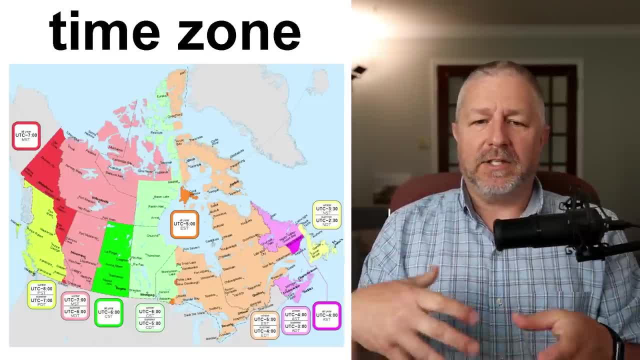 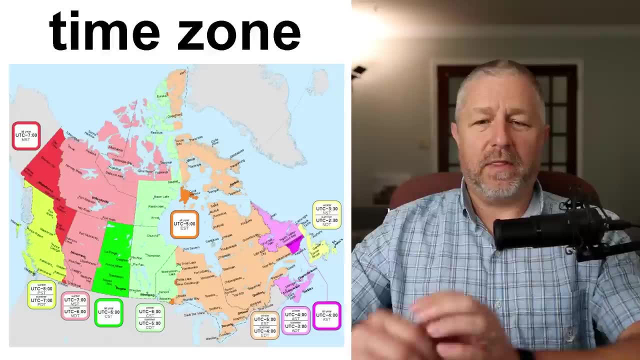 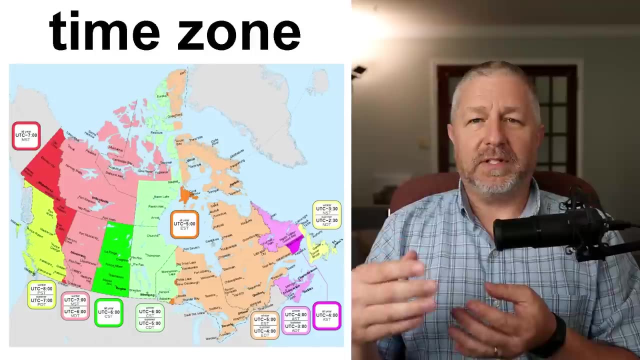 on the other side of the country, in British Columbia, And so there was a three-hour time difference. So when someone lives in a different time zone, there is a time difference. For some of you, it's later in the day than it is here. For some of you living in Europe it's five or six. 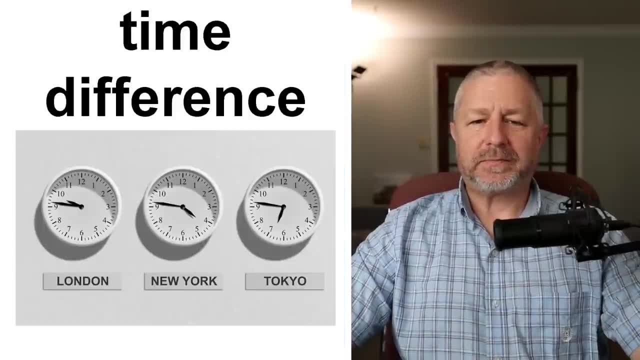 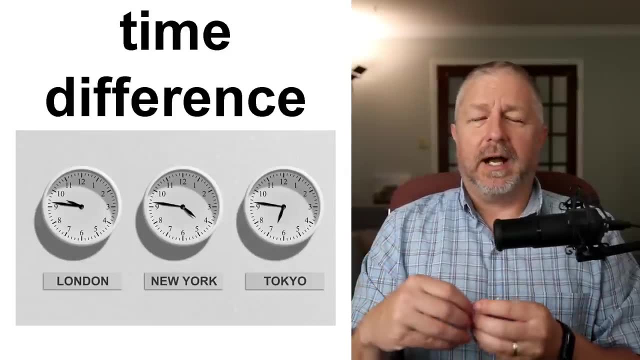 hours later because you live in a different time zone. And then, like I said, we often talk about the time difference. You know what's the time difference between you and me? Um, the time difference between here and France, I think, is five or six. 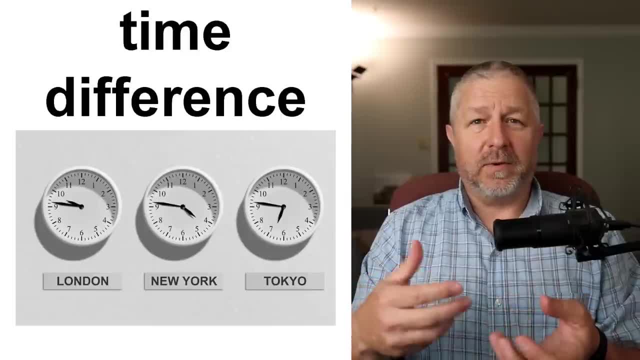 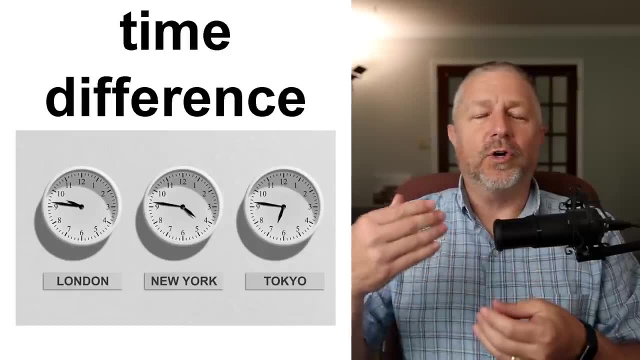 hours right now. So the other day I was talking to my friend in France, uh, and they reminded me that it was evening there, even though it was 11 AM here or early evening there. So when you talk about the time zone that you are in, you often also 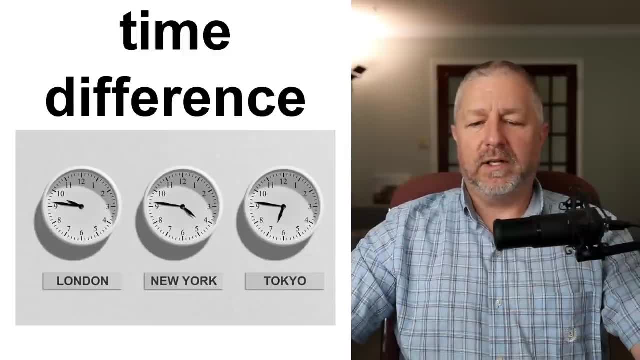 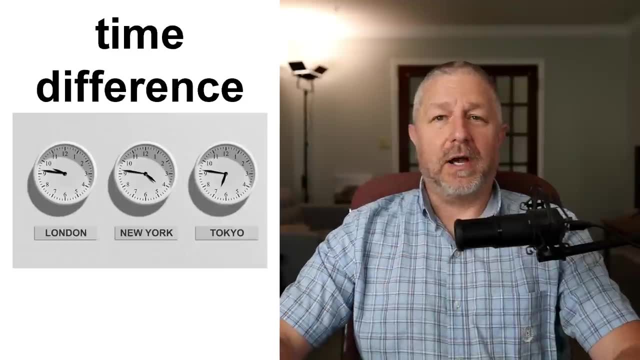 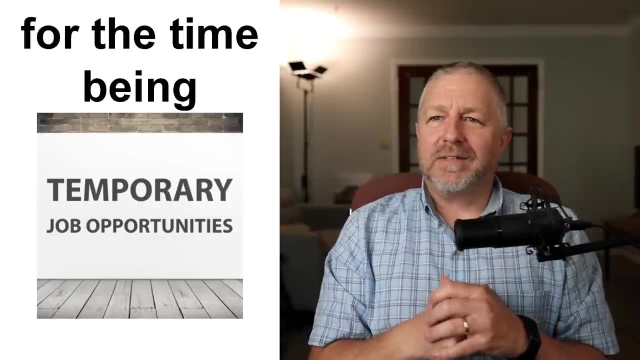 talk about the time difference between where you live and someone else lives. By the way, my time zone is the same as New York. New York is in the same time zone as me, So there's no time difference between me and New York City. So we have a phrase for the time being and we use 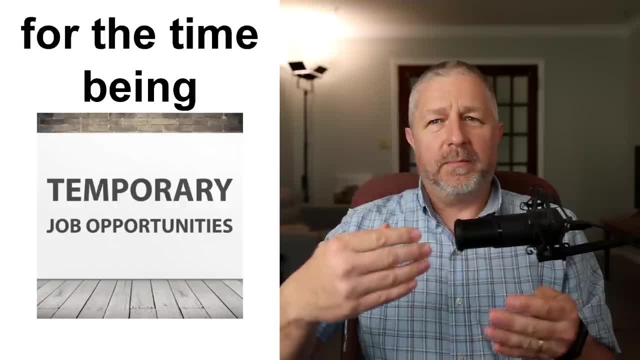 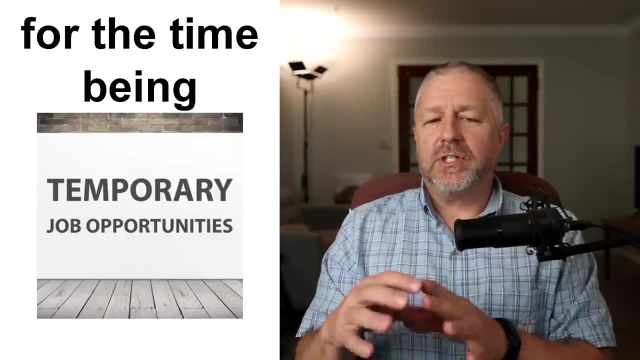 this phrase to talk about something you're doing, but only for a few days or weeks or months. A good example would be if you get a job, but it's just a temporary job while you look for a better job. So you might say this phrase this way: 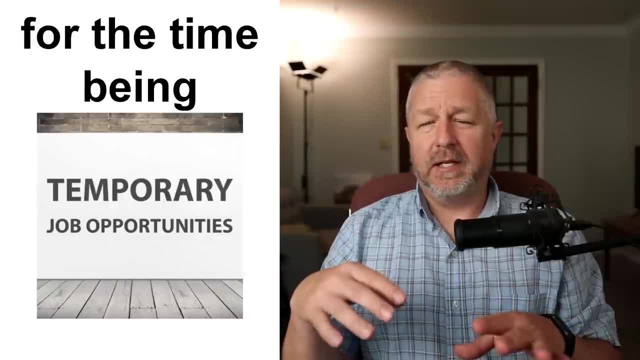 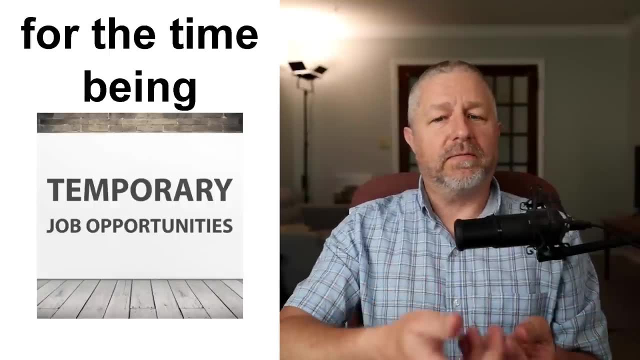 You might say: oh, I'm just working at the gas station for the time being because I'm waiting for a better job. or I'm just working at the restaurant for the time being because I'm looking for a better job. So when you say that you're doing. 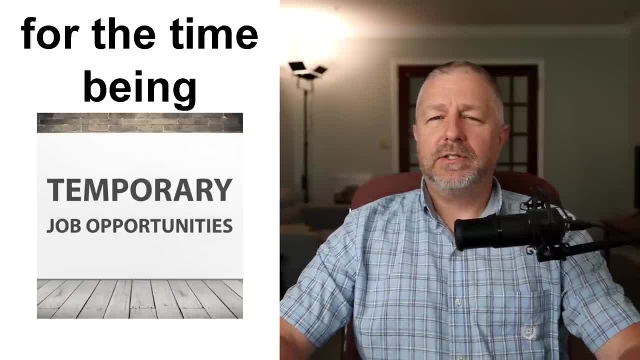 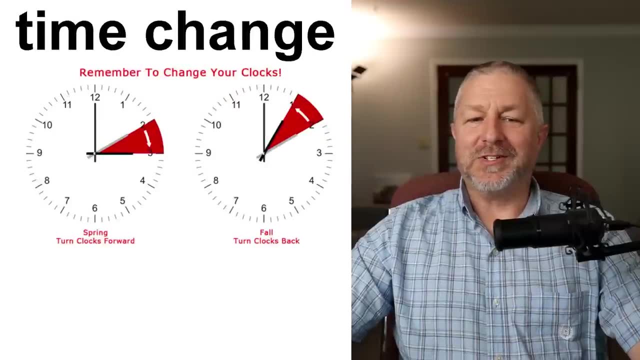 something for the time being. it means you're doing it just for a little while, not forever. Oh, and we also have time change in some countries, So this messes up some of you. This is not nice for some of you, but 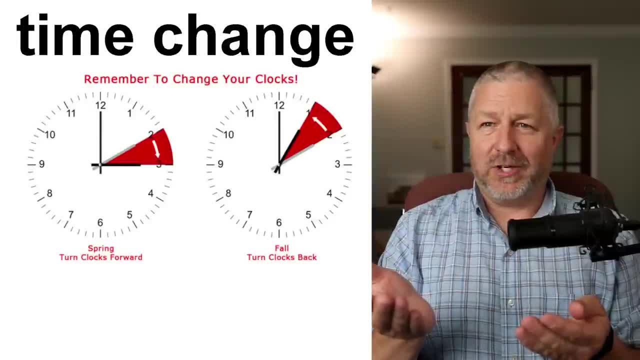 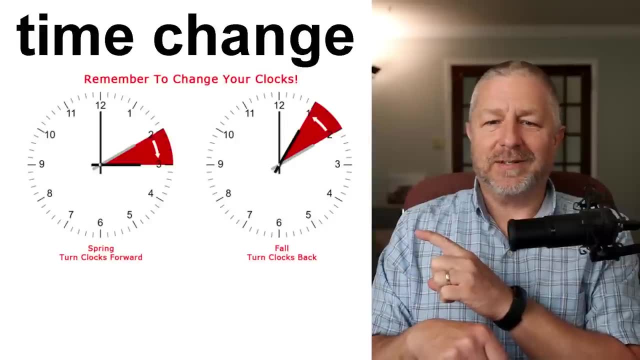 twice of twice a year. we have time change here in Canada. Uh, in the spring it says over there, you turn your clocks forward and you lose an hour of sleep. In the fall, you turn the clocks backwards and you gain an hour of sleep. because we 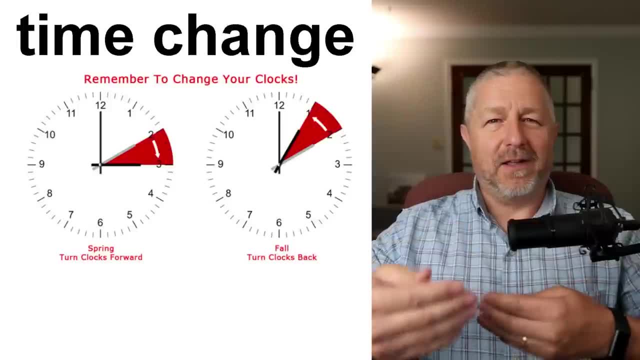 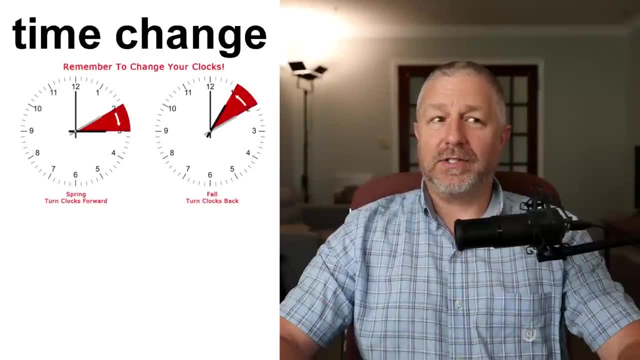 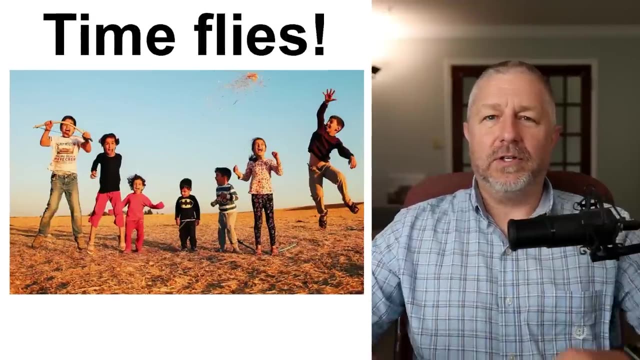 do it at night, and so that's why the time of my live lesson changes every six months. uh, because we have time change and our clocks here, but you maybe don't do that in your country- Time flies, So this phrase is often used when you're having 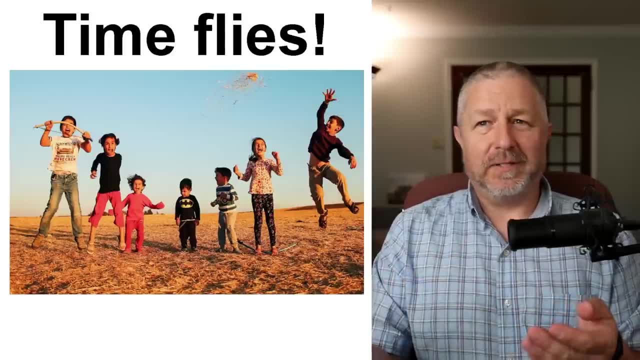 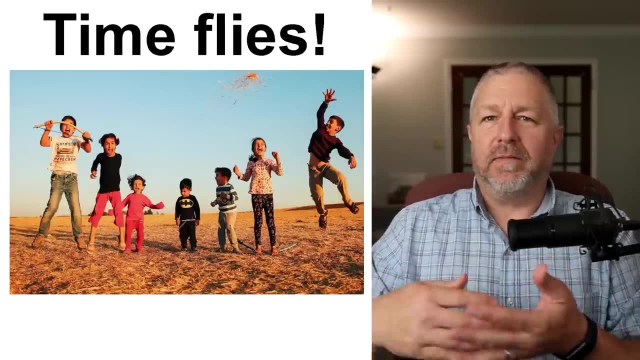 fun. In fact, the phrase time flies when you're having fun means that when you are doing something fun, an hour goes by really quickly. When you're doing something fun, an afternoon goes by really quickly. So we say: ah time. 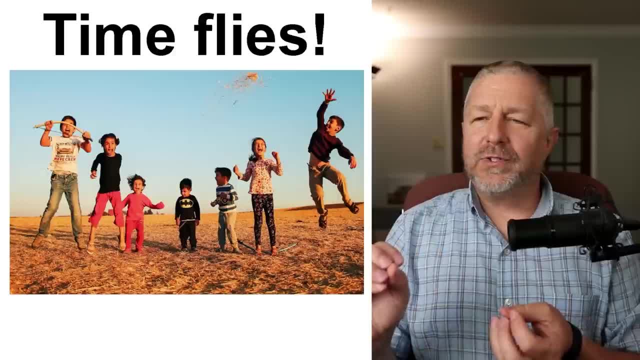 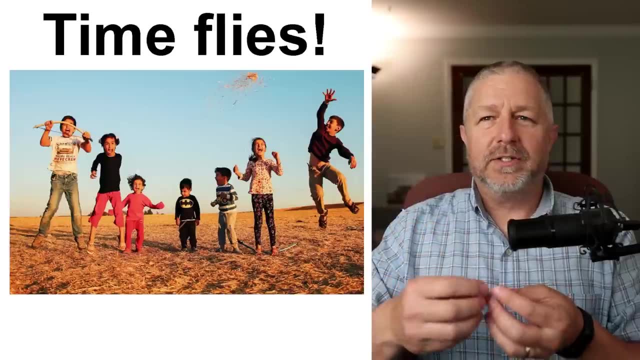 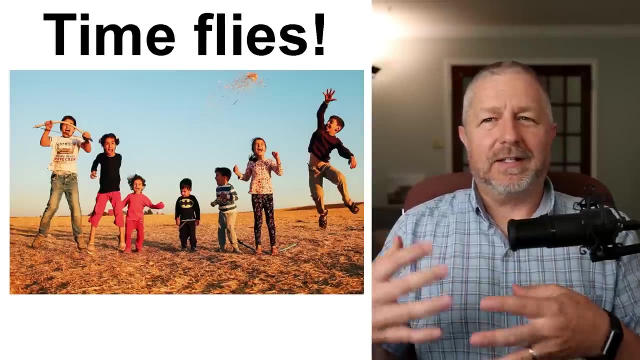 flies when you're having fun, But we also use it to describe. you know. a good example would be when kids grow up really quickly. So maybe you have um children or you have a niece or nephew or you know some children. Um time flies is a statement we say. 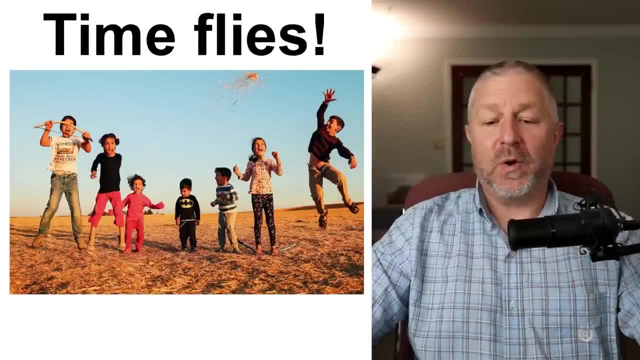 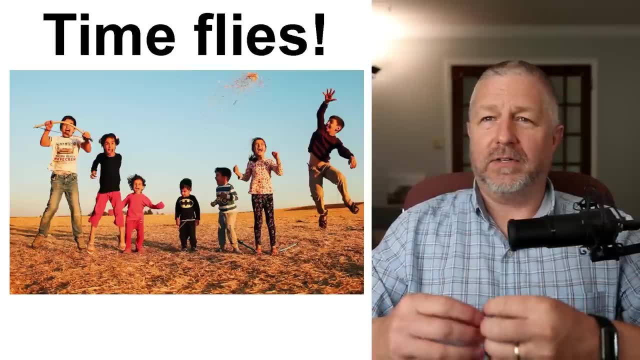 when we realize how fast children do grow up. Um, if you meet your brother and you haven't seen your nephew for a while, and all of the sudden your nephew is the same height as you, You would say, oh wow, time flies. An expression. 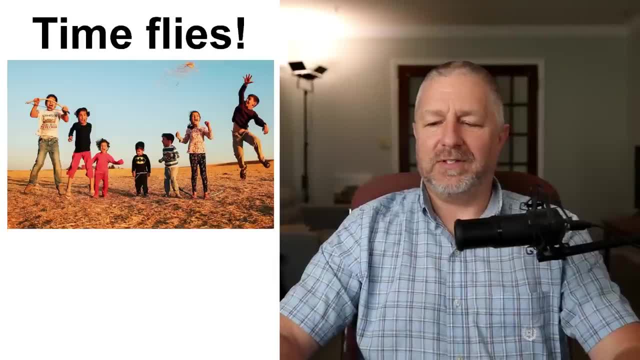 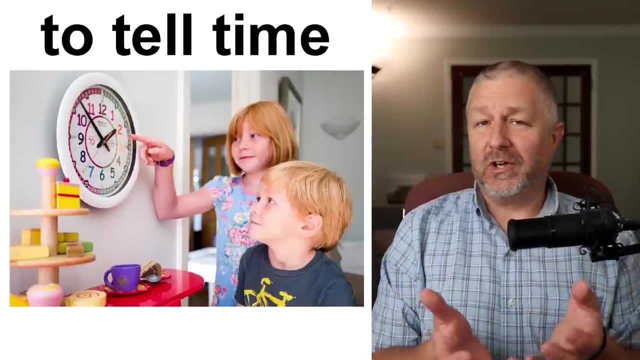 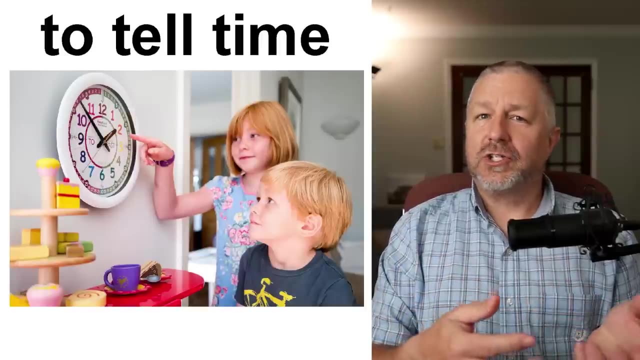 of how fast it sometimes feels like time is going To tell time. So the ability to look at a clock and say what time it is is called. we use the verb to tell time. We teach children how to tell time. I can tell time, okay, I'm able to look at. 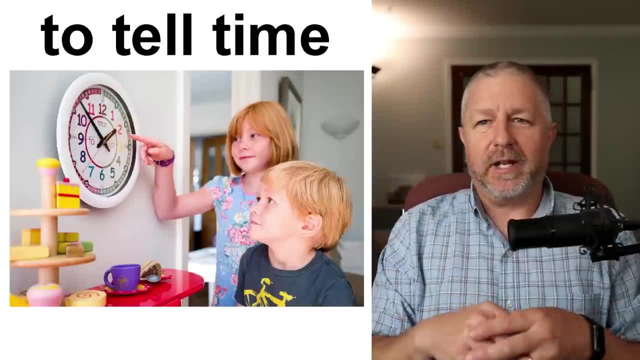 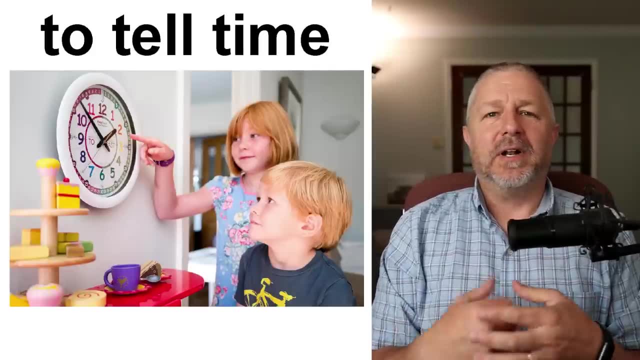 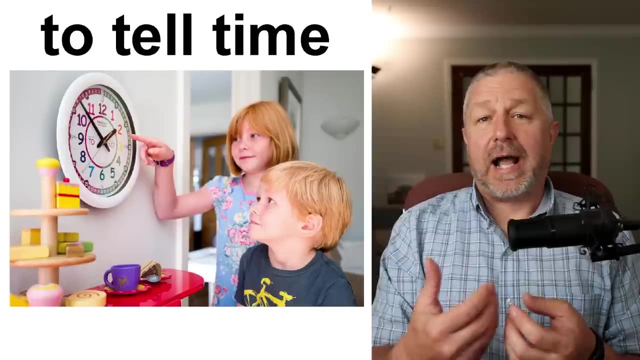 my watch and I'm able to look at any clock in the world, and I should have done some research before the lesson. But often children at age four or five or six are taught to tell time. They're taught how to look at a clock or watch and be able to. 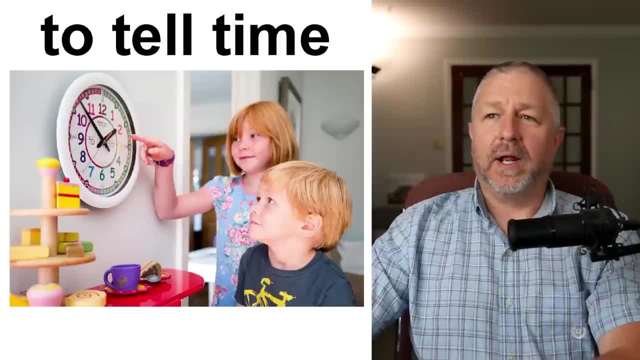 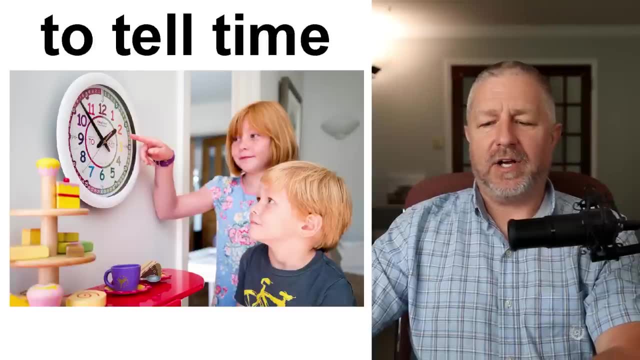 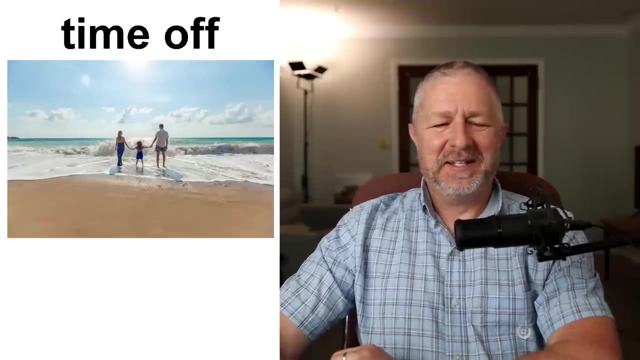 say what time it is. So I think when I was in kindergarten- age five or grade one- age six, I think, somewhere around that age- I learned how to tell time. I can still- and I still know how to do it. Time off- This is something that we use, This is a phrase we 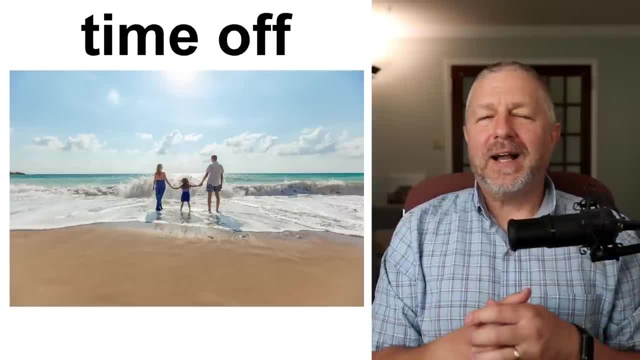 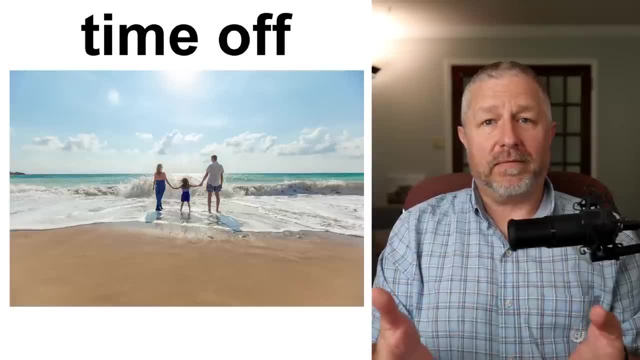 use to describe when you are not working. Um, someone might have time off during the summer. Teachers in Canada and in the United States have time off in the summer. Right now I'm on summer vacation. I have time off, You might know. 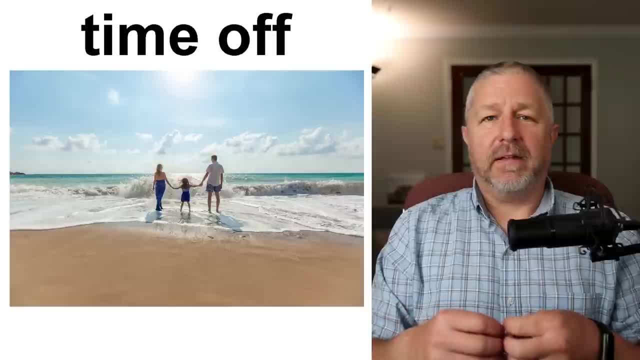 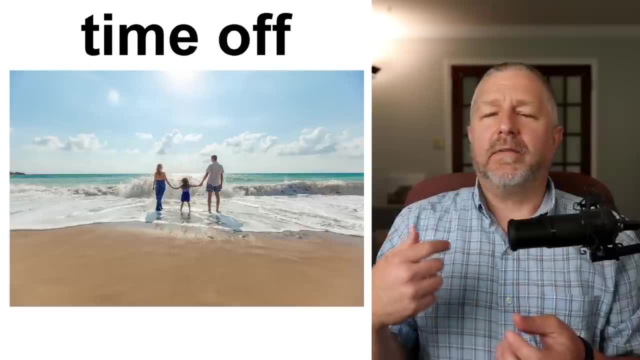 someone who works at a factory and they get five weeks of vacation a year. That would be nice. You would say, oh, when's the next time you have time off? Oh, I have time off in a few weeks. I'm going to take two. 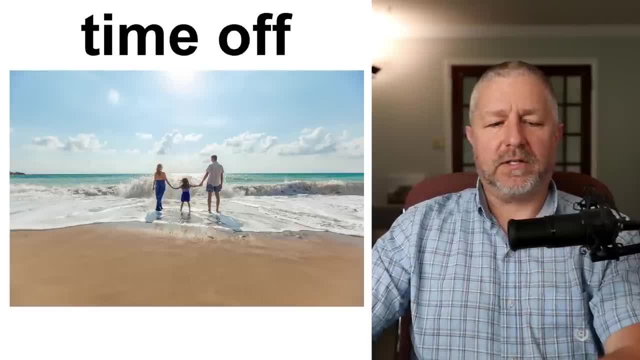 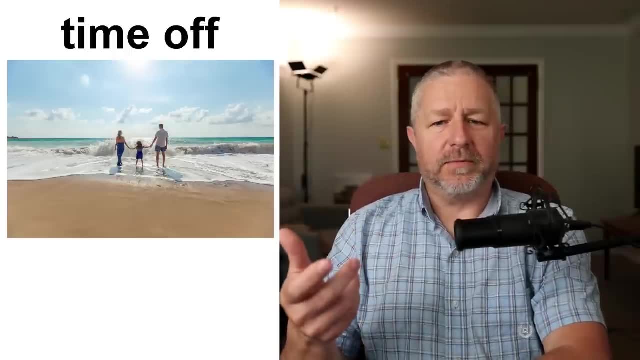 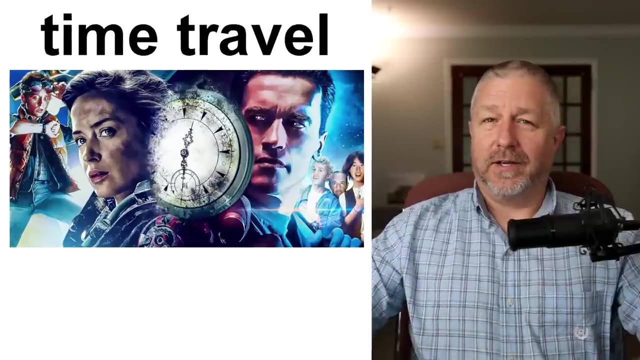 vacation days. So time off refers to any time when you are not working, but you can also use it to talk about school. You know you can take time off from school to do something else- Time travel. So I do like science fiction novels and 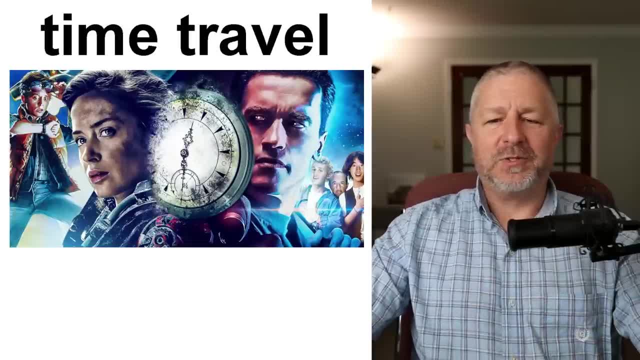 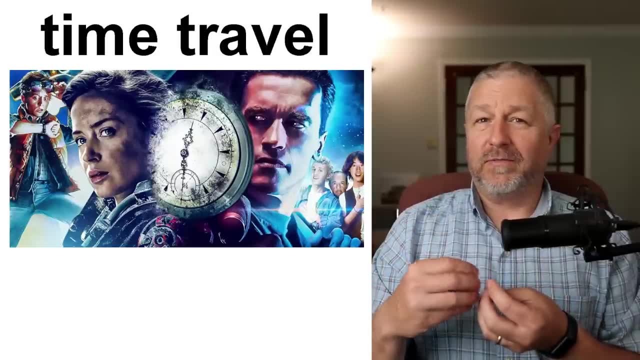 I do like science fiction movies and I do like time travel. It's kind of fun to read a story where they travel in time, So you either go forward in time or backwards in time. Um, so these are all pictures of different I think. 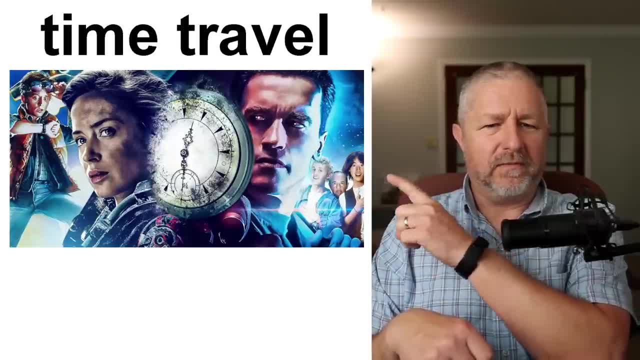 movies I think we have Back to the Future, at the very far side, and at this end we have Bill and Ted's Excellent Adventure, I think. Then I'm not sure what that movie is. Um, that's the one where Tom Cruise keeps going back in time all the. 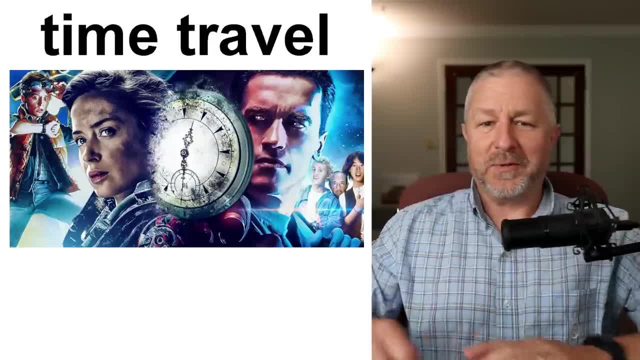 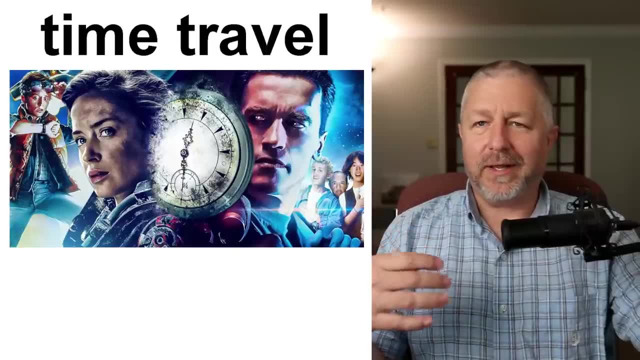 time. and then I'm not sure about the Arnold Schwarzenegger. Is that Arnold Schwarzenegger? I don't know. Anyways, when you travel through time, you can travel forward in time or backwards in time and, by the way, time. 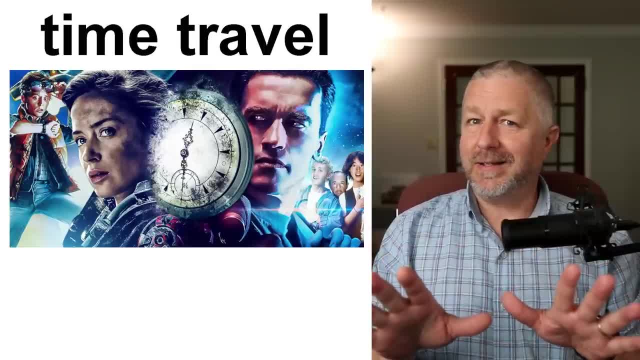 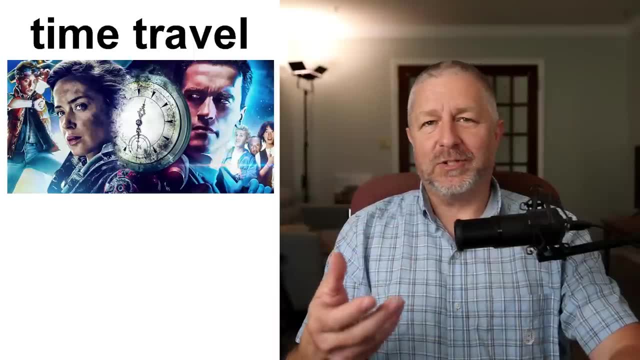 travel doesn't exist. At least we don't think it does. Um, but we have no evidence that it is possible. It's just something you read about in a science fiction book or see in a science fiction movie Time out. So if you watch sports, 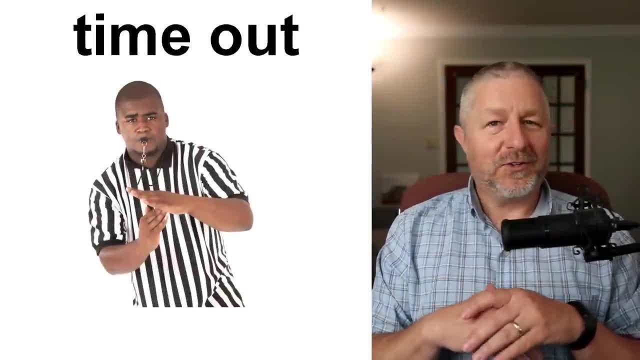 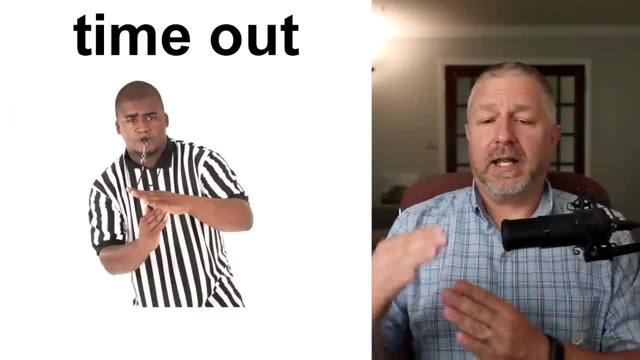 you know about time out. If you have kids, you might also know about time out, and I'll explain the difference. In a game like basketball, the coach or a player can ask for a time out. A time out is when the game stops and the coach and players. 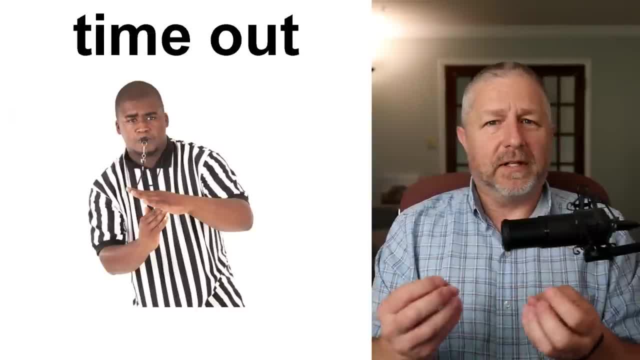 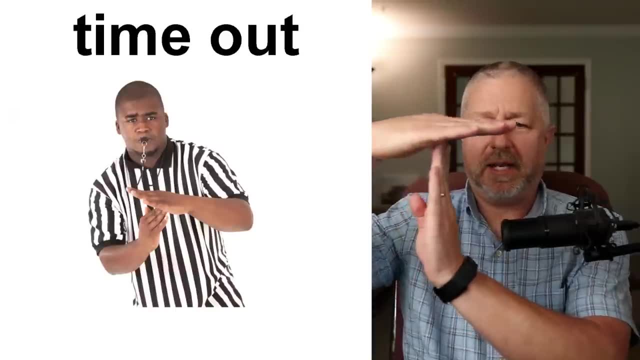 can talk for 30 seconds or a minute- It's different lengths in different sports, Um, but this is what the ref will do or what the coach might do, Like time out, time out. They're making the letter T Meaning I would like the game to stop, so 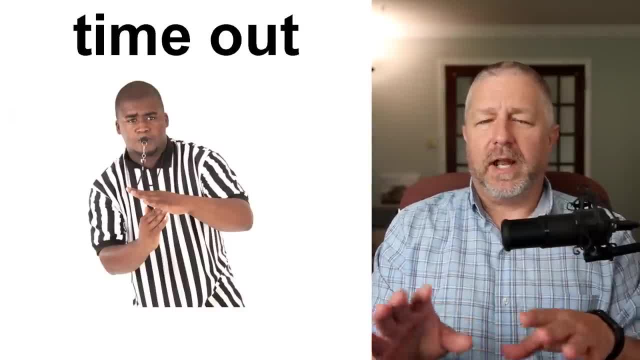 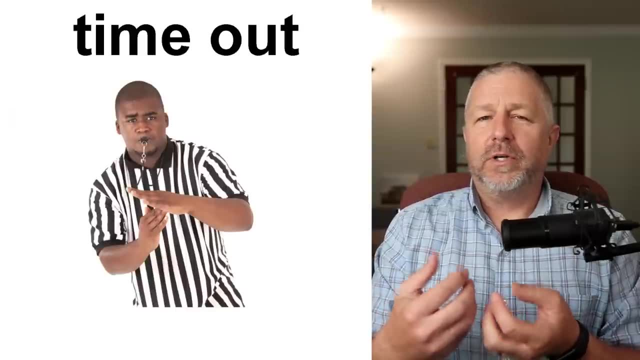 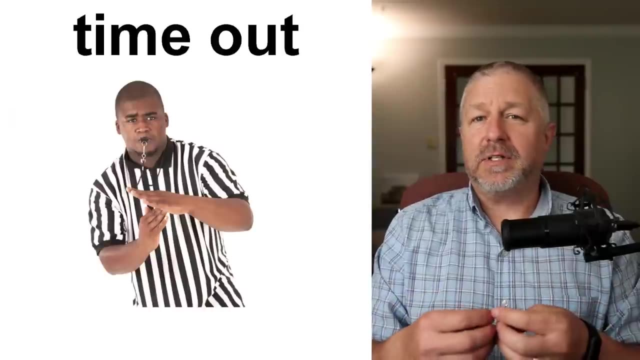 I can talk to my players, Um, and I think you can only use so long on which sport you're in. We also use this for when we're teaching children how to behave. If a child doesn't do what a parent asks them to do, sometimes the parent will give. 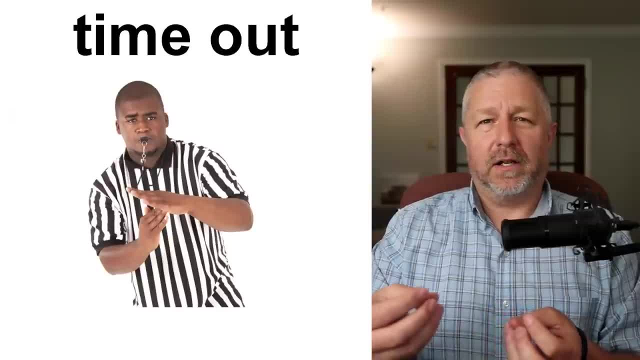 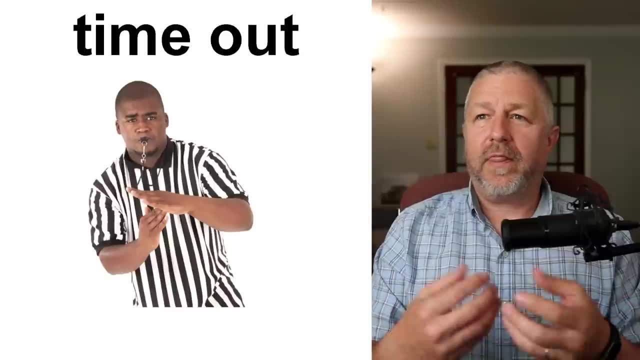 the child a time out. They might have to sit on the stairs for a minute, or they might have to sit on a chair in the kitchen, and they're not allowed to go anywhere while they think about what they've done. So a time out is a common way to. 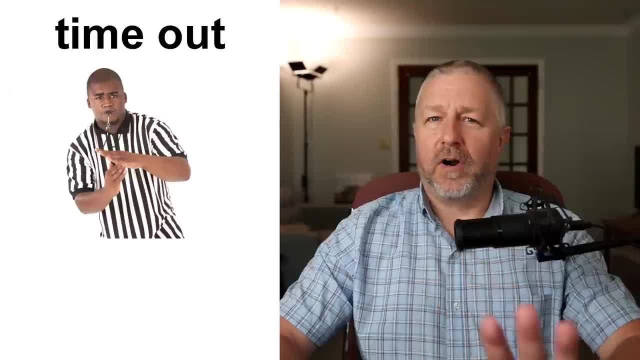 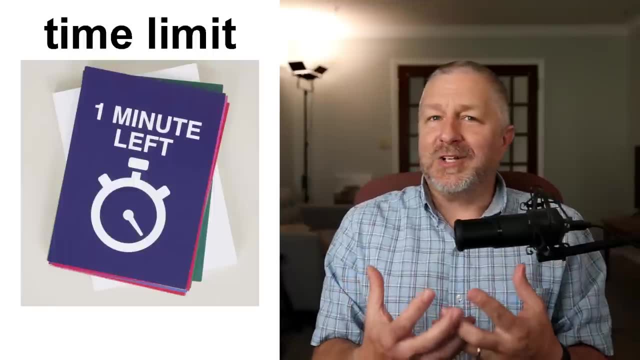 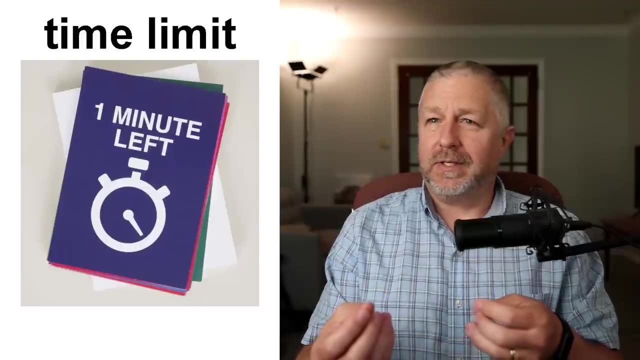 train children, To teach children how to behave, And I think that's a common way to teach children how to behave, but it's far more common to use this when talking about sports Time limit, So this is something that can cause stress. The other day, I had to renew my driver's license. 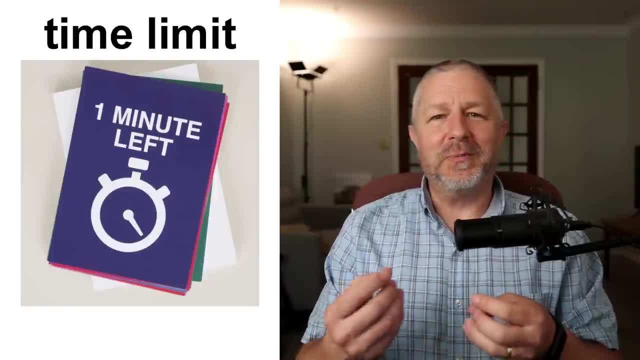 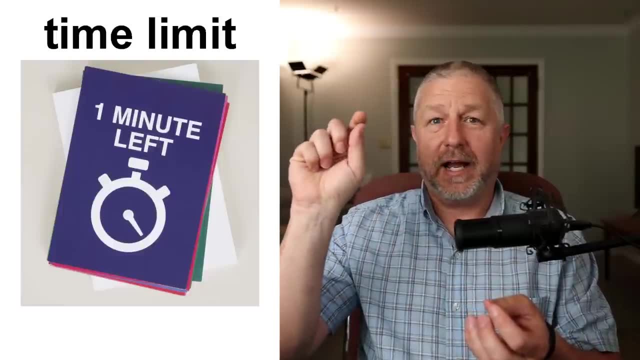 because it's July, So somebody had a birthday. but I had to renew my driver's license and I could do it online. but when I started the process there was a timer saying I had 10 minutes to finish it. There was a time limit. So when something has a 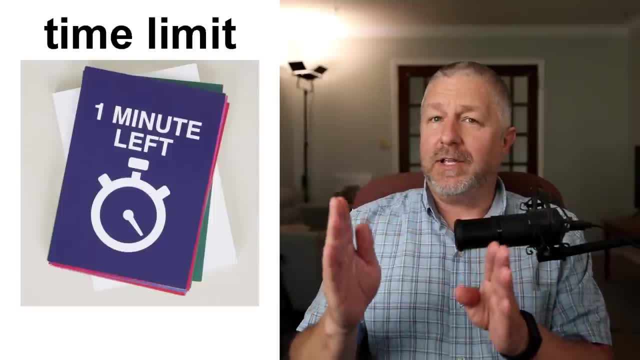 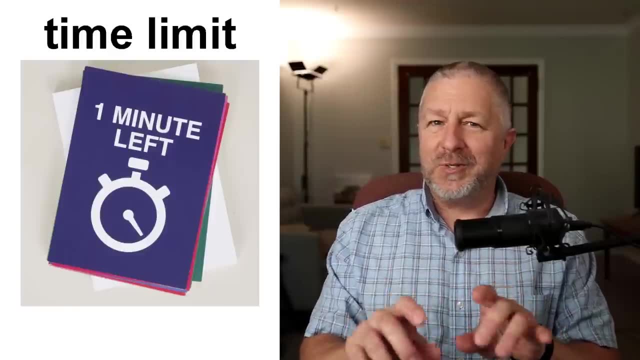 time limit. it means a clock is running and you only have so much time to do something or complete something. So I very quickly tried to do all the renewal stuff and it took me quite a while- Not 10 minutes- but it was a little stressful. 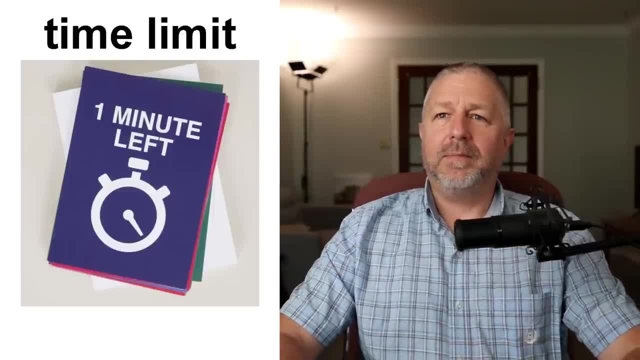 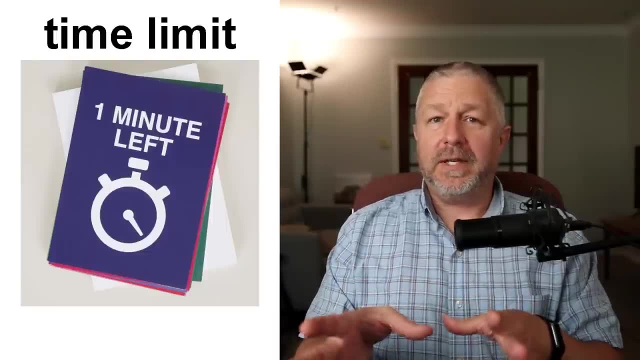 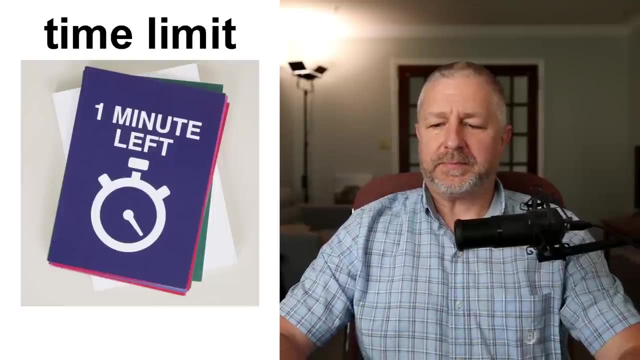 that there was a time limit. Sometimes there's a time limit. maybe something's on sale and they'll say: for a limited time, that means there's a time limit, That means you only have a few days to buy that item that is on sale, A timeline. So 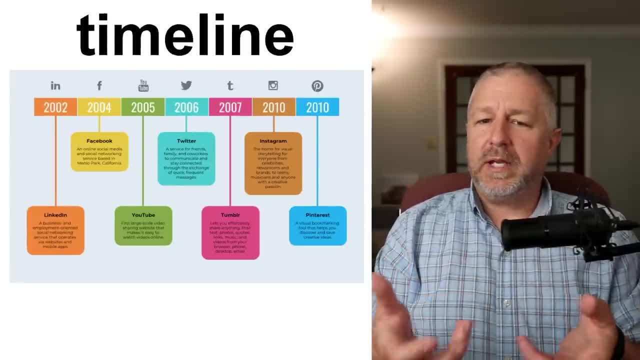 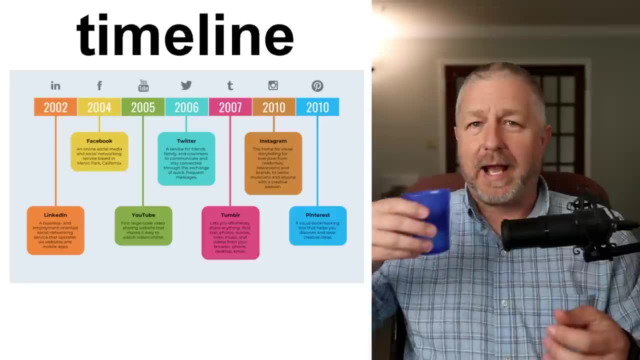 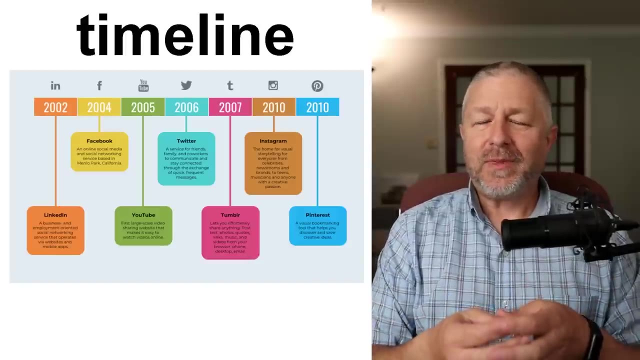 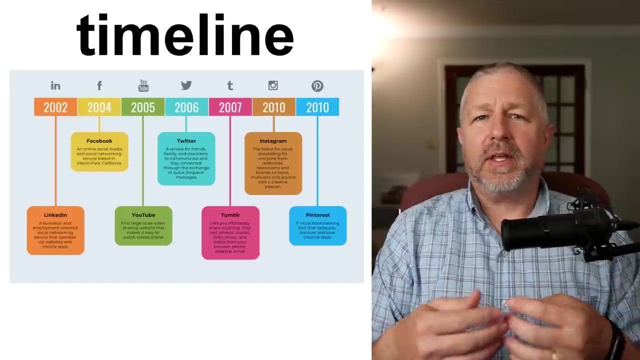 this is the timeline of different social media apps. And a timeline- is this really nice visual graphic of what has happened over time? If you ever studied history in school, you have seen or made timelines. So they might say: create a timeline about the history of Canada from 1800 to 1900.. So 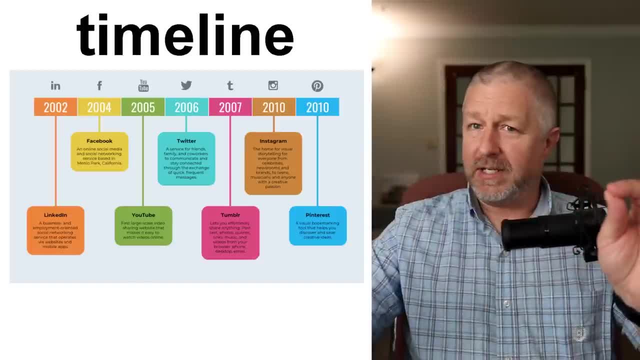 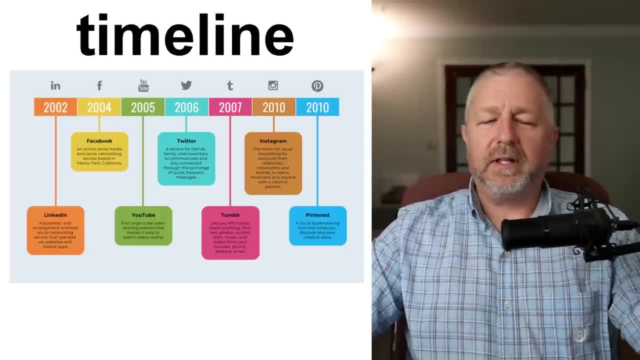 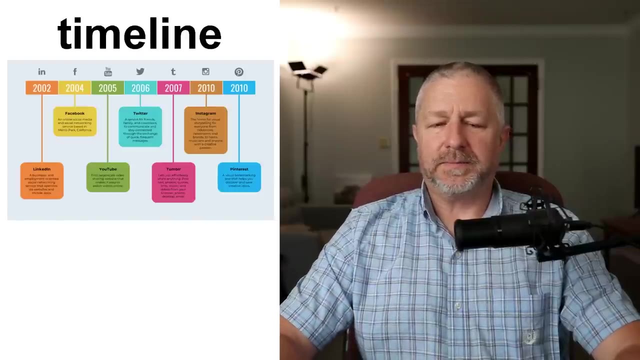 you would draw a line and you would put the date 1800 and 1900, and you would put important events on the timeline and describe each of them. So something that you commonly see in school but you also might see when you're reading a magazine or other news article: Time lapse. 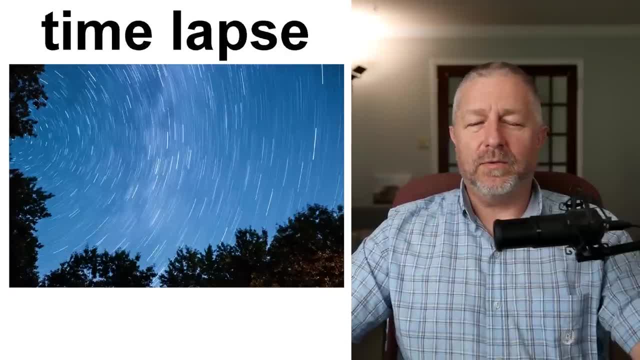 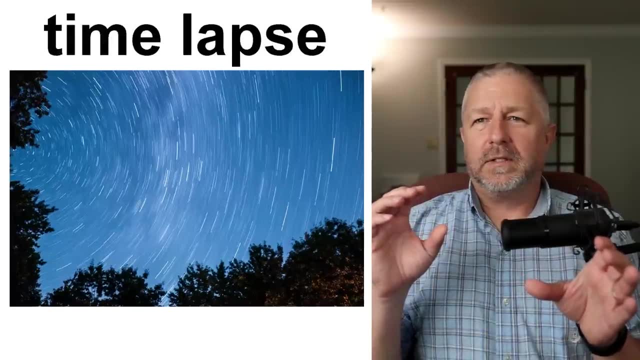 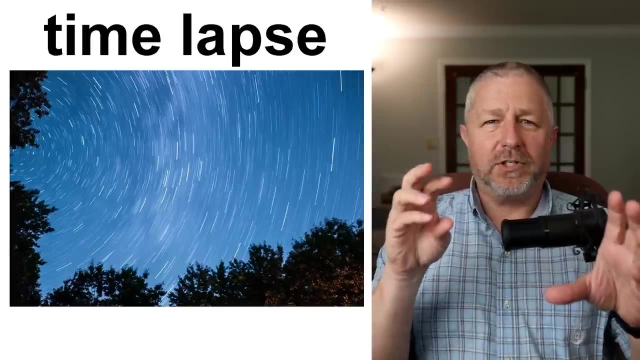 So a time lapse is a technique that you use when taking a photo where you- yeah, I gotta, I. I think I'm better off describing it with video. So a time lapse is when you take a picture, maybe every minute, and then you put all those pictures. 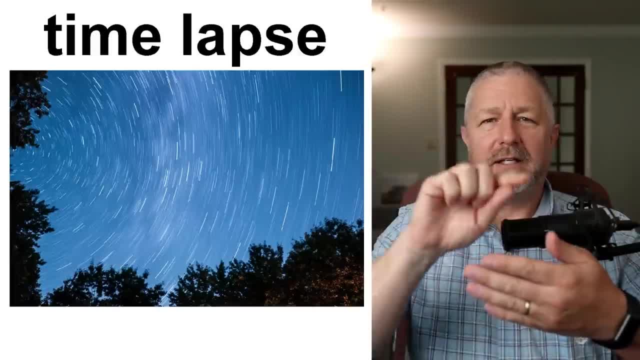 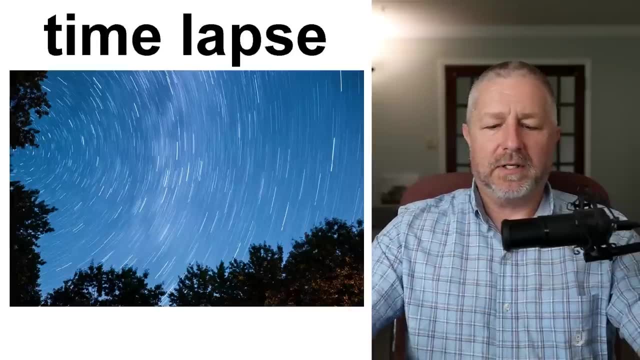 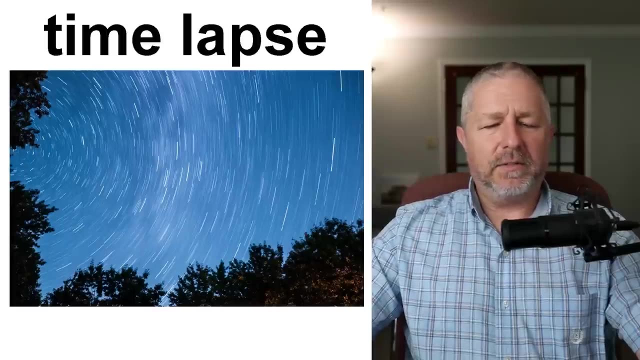 together and then when you play them, you can see it move. Let me get the dictionary definition of time lapse, because I think there's a couple different meanings of time lapse. Meaning of time lapse: So the technique of taking a sequence of pictures at set. 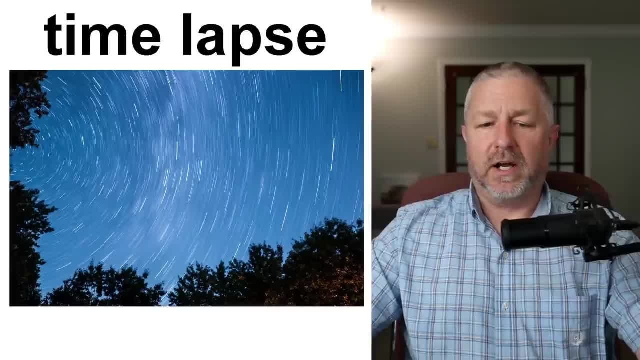 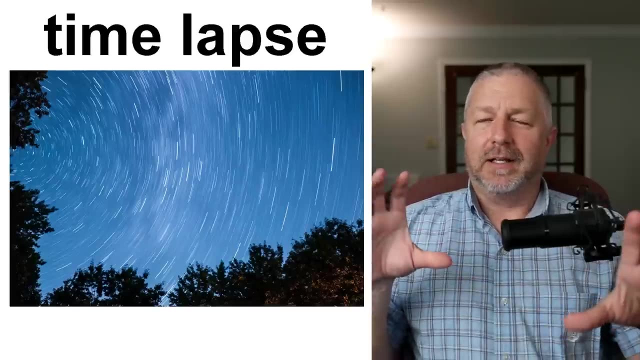 intervals to record changes that take place slowly over time. Frames can then be combined and watched as a video to at normal speed, showing the action much faster. So hopefully that made sense, but I think you understand what a time lapse is. It allows you to 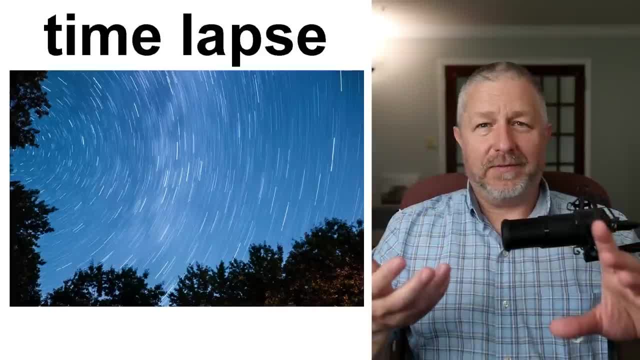 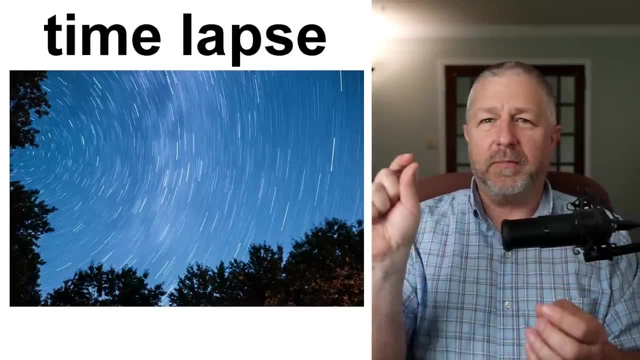 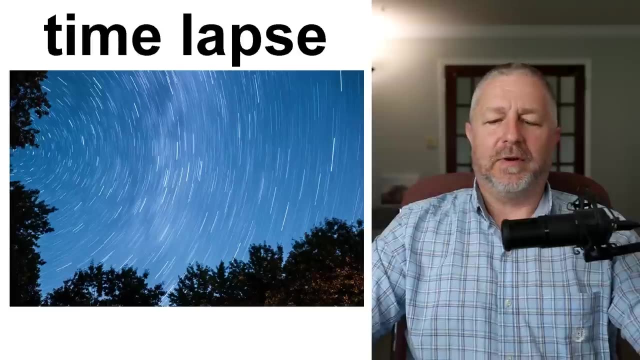 like if I was to do a time lapse of this lesson of me here and then you would watch the whole lesson in one minute and it would just be one picture of me every minute for an hour, so it would end up being 60 seconds long. If it was 60. 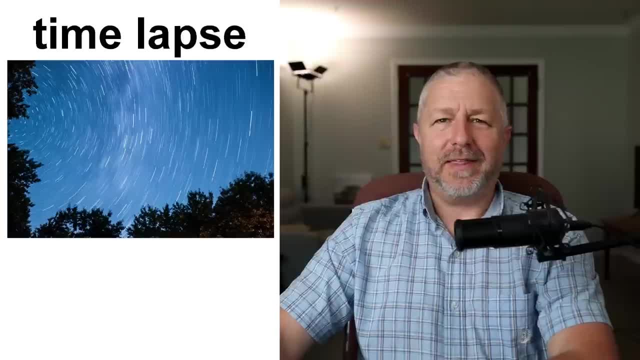 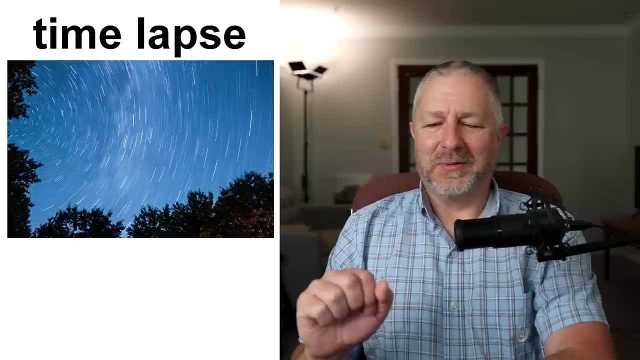 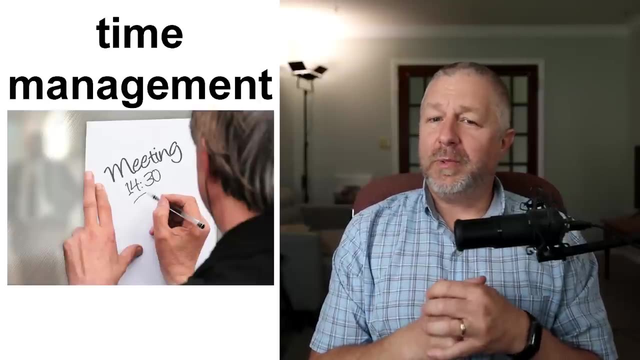 frames per second. Hopefully I explained that well. I'm not sure I did, but I think I always. I'm always- allowed one slide during the lesson that I don't explain well, and then you can figure it out on your own Time management. This is something that you want to be. 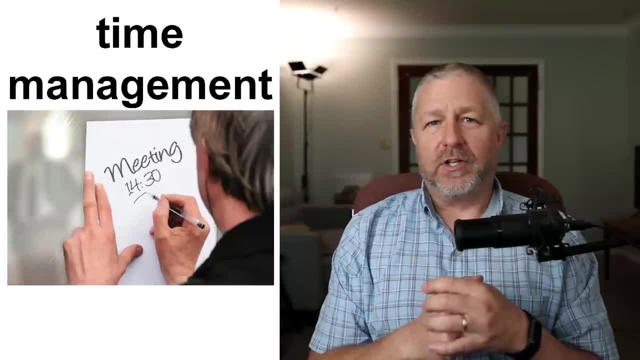 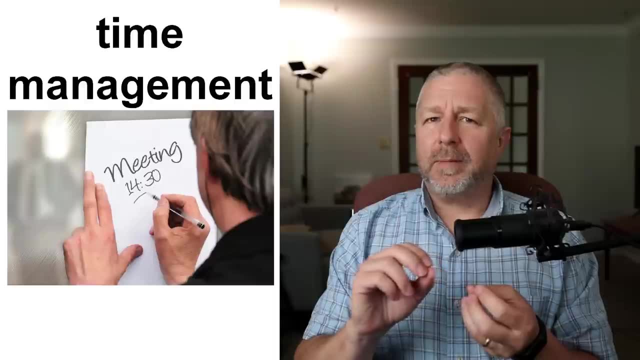 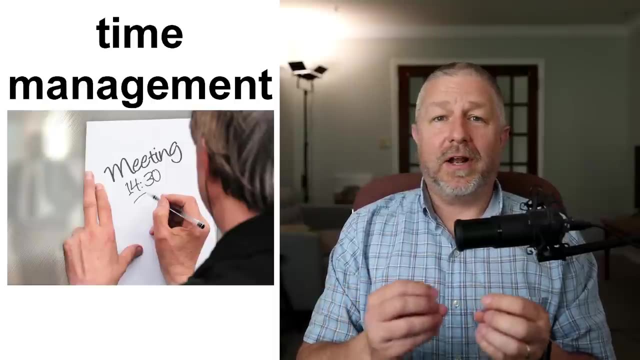 good at It's a good skill to have. When someone has good time management skills, when they're good at time management, It means they are really good at planning things. If your boss isn't really good at time management, it's probably not a fun place to work. Things probably happen. 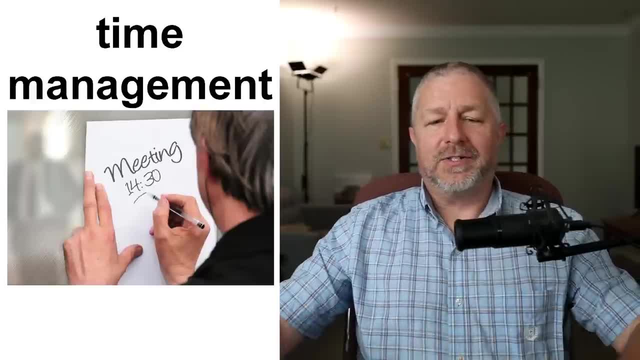 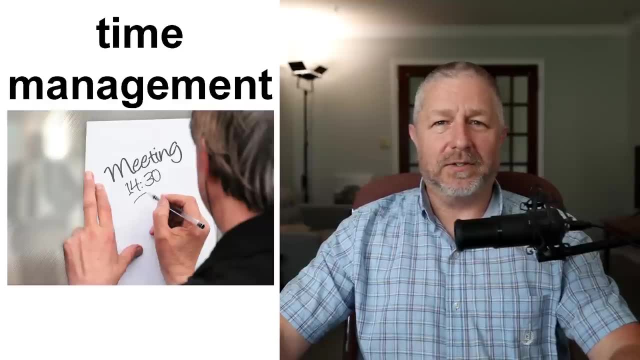 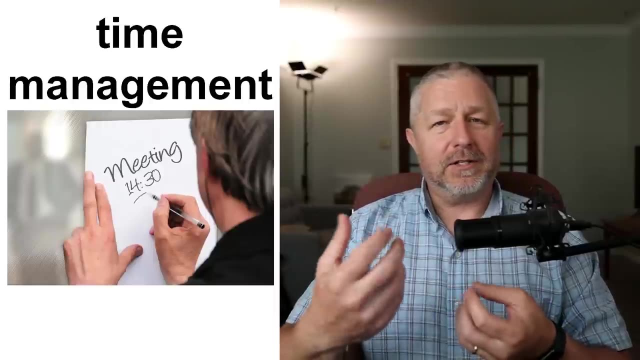 late or early or not at all, and so it's nice when you work with people or when you work for people who have good time management skills, They write things down in a calendar. They write down the time and date of things. They communicate well with people Like don't forget the meeting. 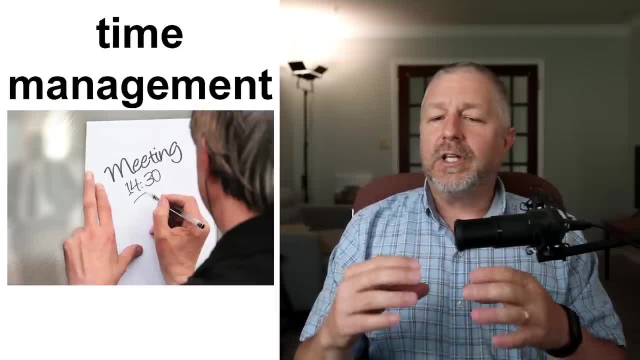 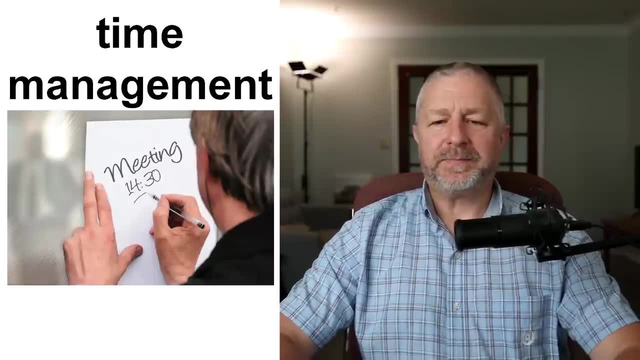 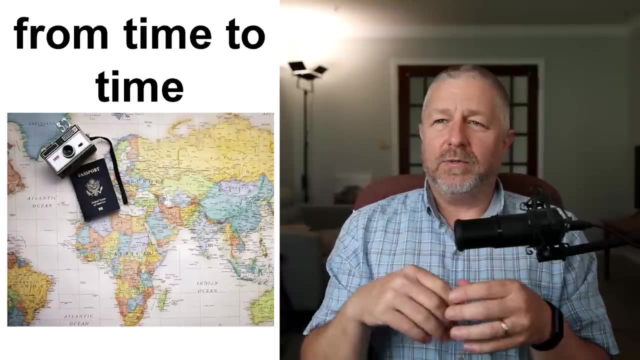 starts at nine. They have really good, a really good ability to manage their time and if they're in charge of other people to manage the time of others, Time management From time to time. So this phrase is used to talk about something that you don't do very often, Something that you do every. 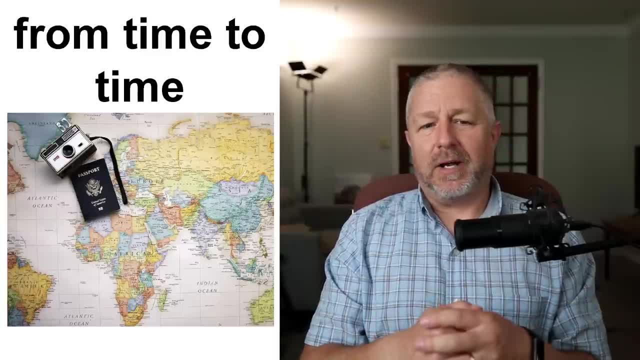 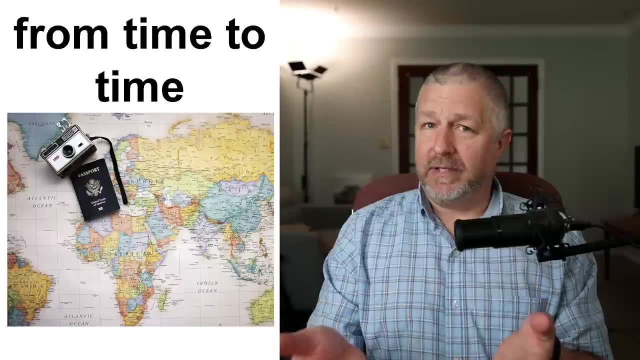 once in a while. That's another English way to describe it. So here's how I would say this: Most people, from time to time will travel. They don't travel every day, They don't go on vacations every day, But from time to time they'll go and 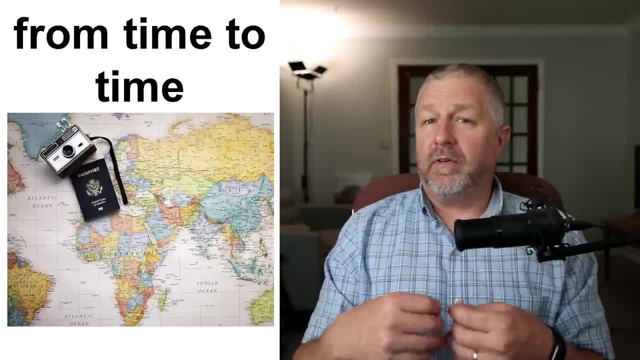 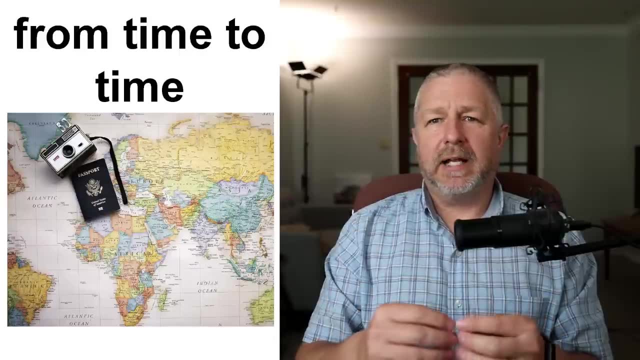 visit someone far away. Jen and I go and see a movie from time to time. That doesn't mean we go and go every weekend or every day or every month. It just means that every year we see about four or five movies, So we go. 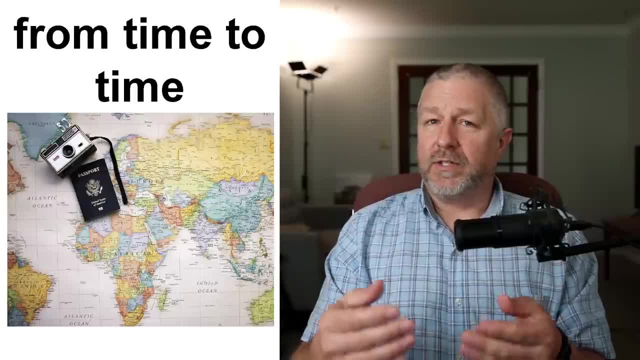 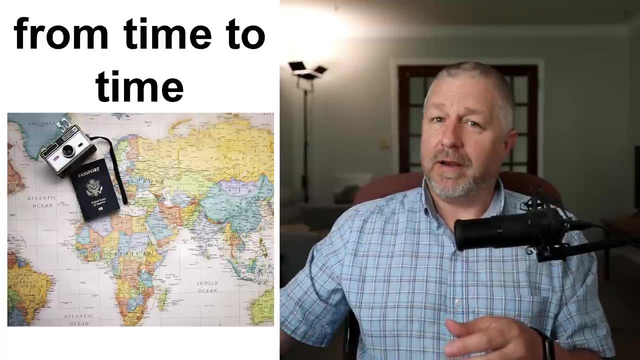 see a movie from time to time. Some of you watch these English lessons from time to time. Some of you come every week, But some of you just watch one from time to time. You don't watch one every time. I do one. Sorry, I have a little tickle in my. 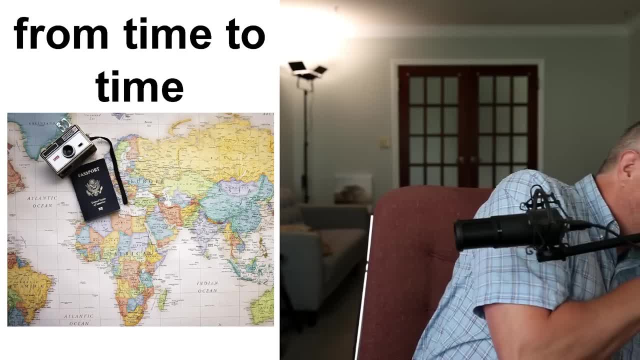 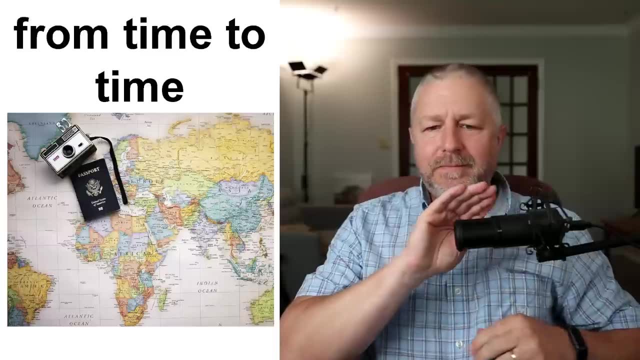 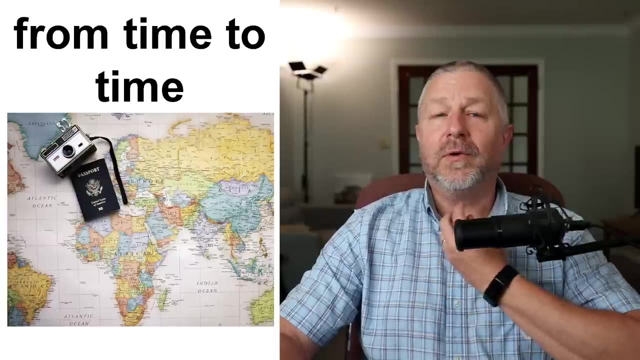 throat. I'm going to go over here for a minute. Excuse me, I should cover the mic. Sorry to do that in the middle of a lesson, But sometimes when you talk your voice gets a little scratchy, It's from all. 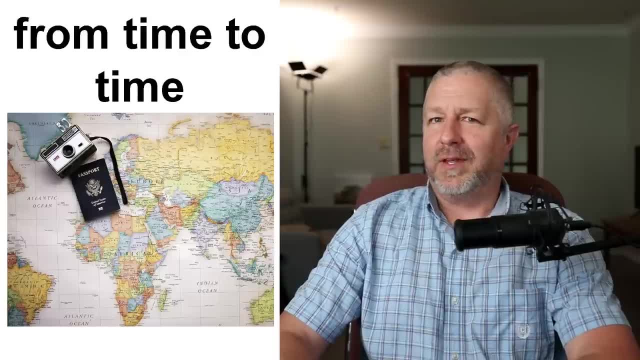 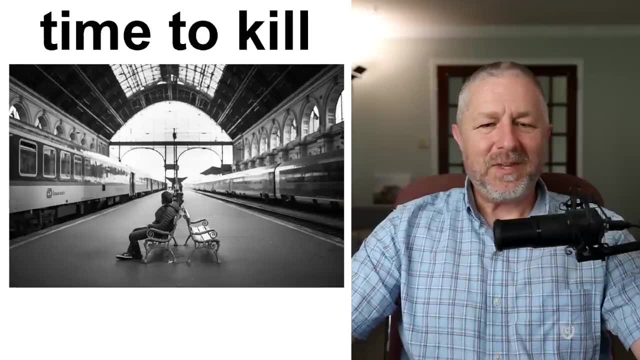 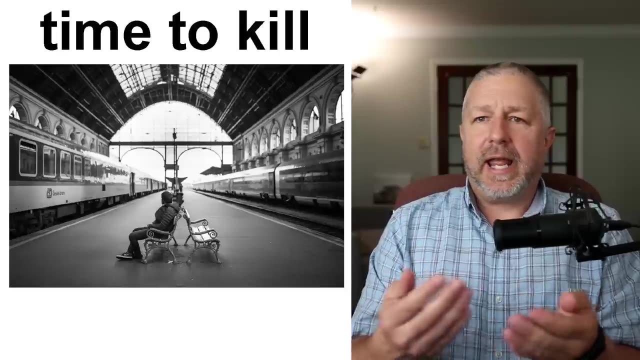 the yelling I did at my birthday party, Or did I? Maybe my birthday party is next week, We'll see Time to kill. When you have time to kill, it means you are waiting your son's somewhere and you really can't. you don't have anything else to. 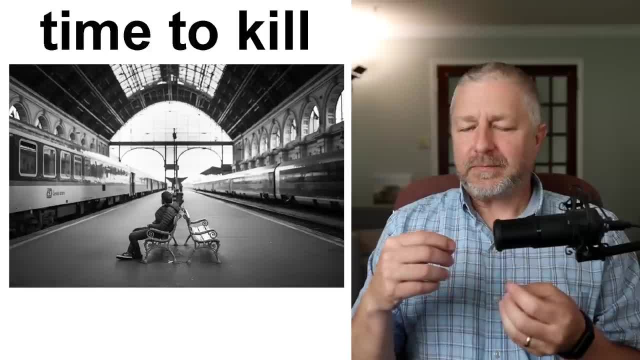 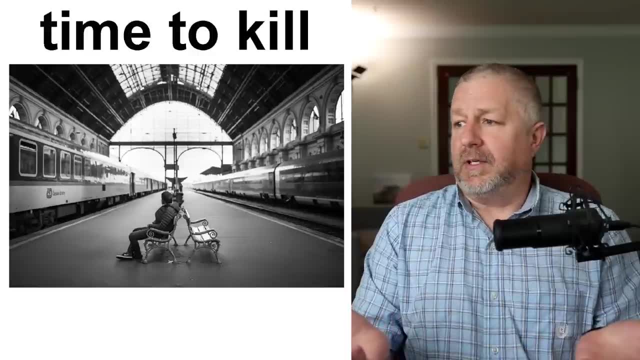 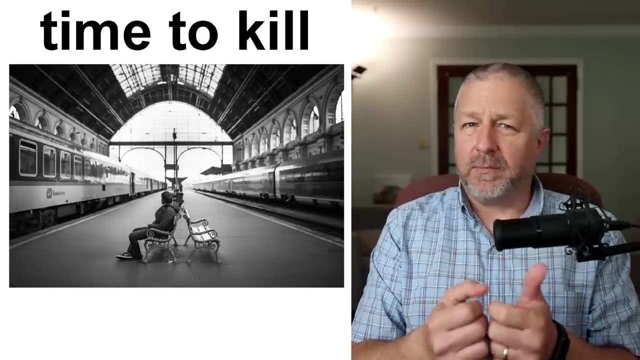 do. The best example I can give is this: Sometimes my kids have an appointment, So I'll bring them to the dentist and then I have time to kill While they go see the dentist. I have time to kill, So usually I go on my phone. I reply to some comments. 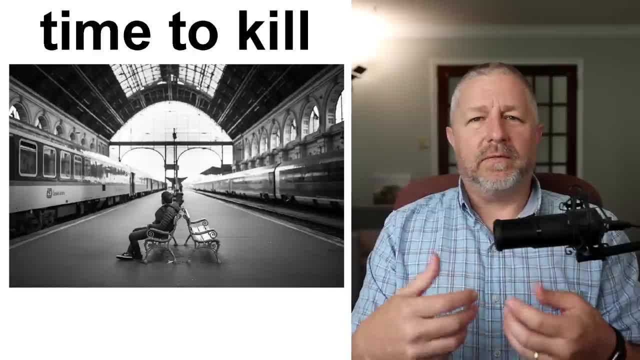 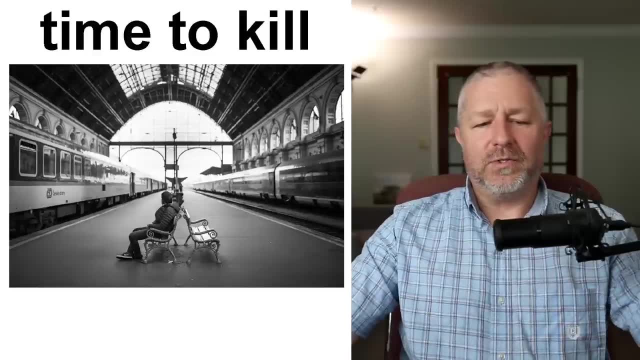 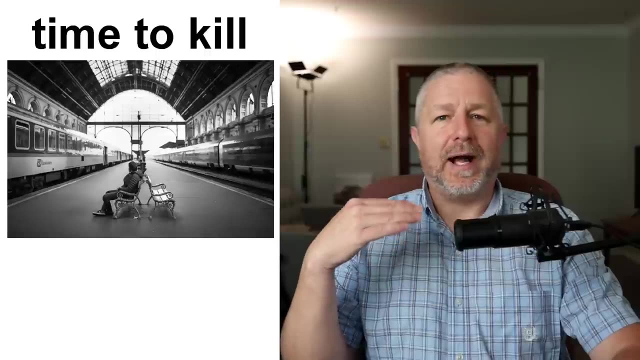 I might run and get some groceries, because when you have time to kill, it's nice to fill that time. There's another phrase: that time with some errands or to get something done. So if you are ever a good example too would be if you're traveling and 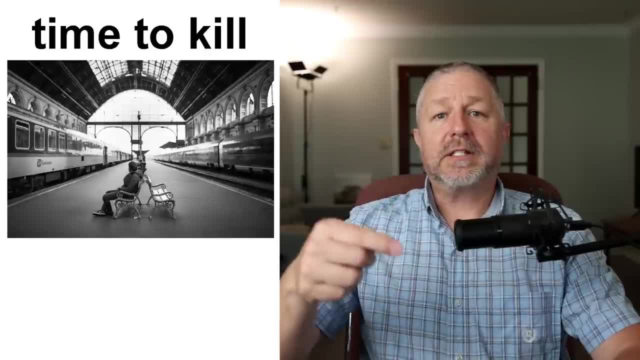 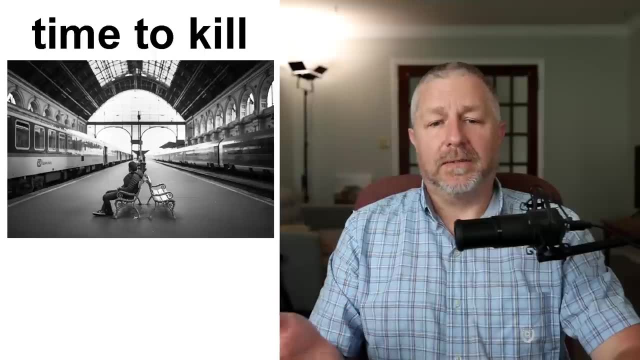 if you land at one airport and then your next flight doesn't leave for four hours, you would say, oh, I'm gonna have four hours to kill, I'm gonna have time to kill. So, basically, you can sit at the airport and study English. That's what you. 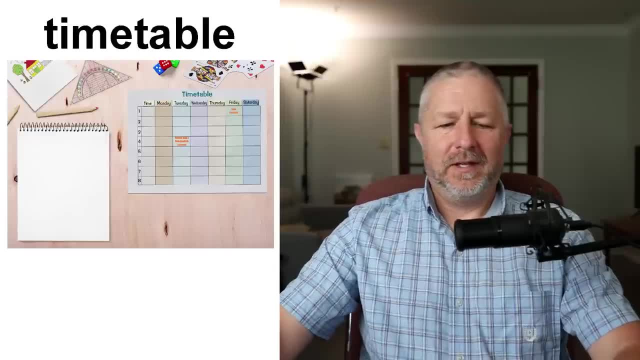 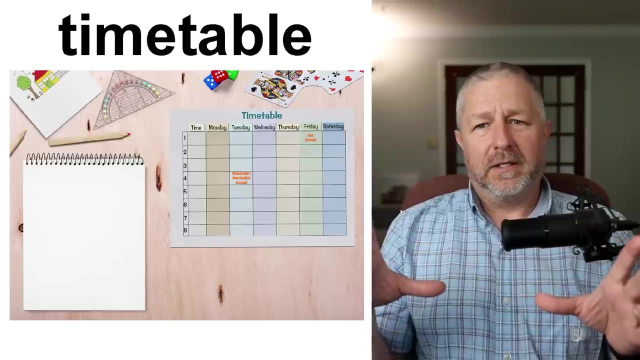 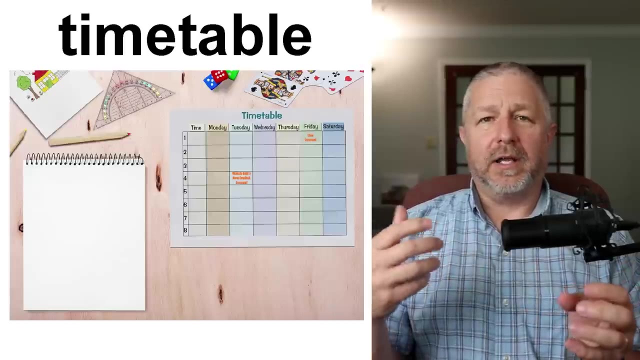 should do when you have time to kill A timetable. So a timetable is basically an outline of your week with important things on it, And it's mostly used, at least in Canada, where I live, when talking about students. Students will receive their timetable at the beginning of a. 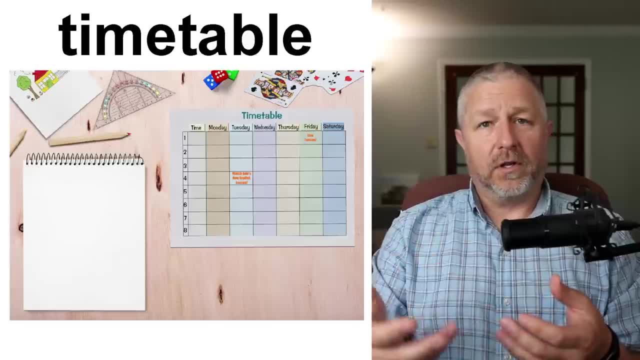 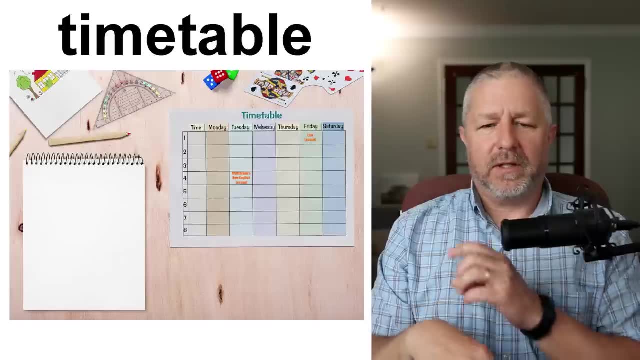 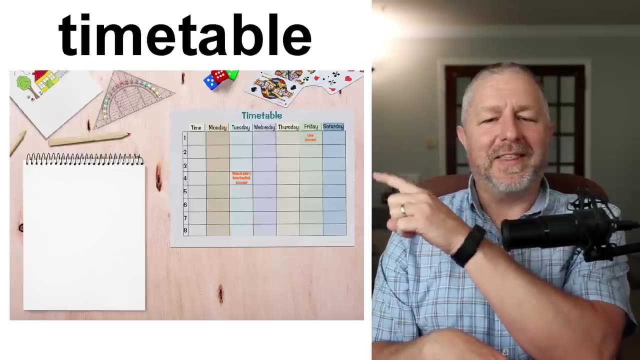 school year. If they are in a high school, or if they're in college or university, The timetable will show what classes they have on certain dates. This timetable, I think, says something about Bob. watch Bob's new video and live lesson. I think that's what I put those words on. 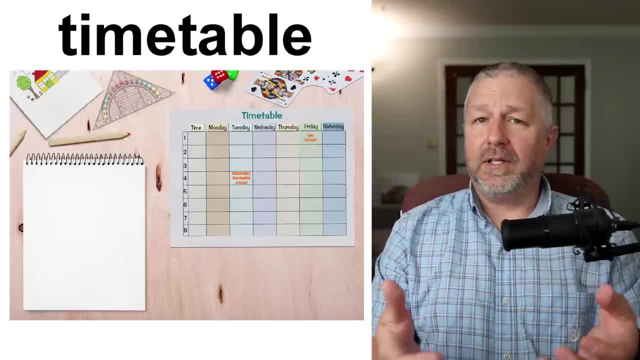 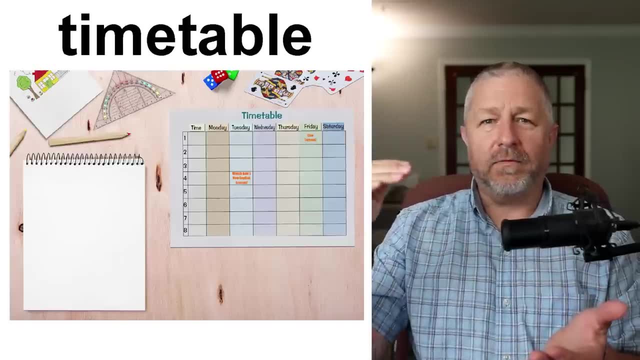 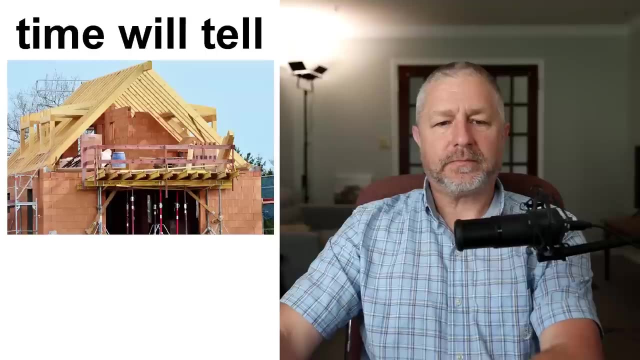 there, But a timetable again, very commonly used when talking about students And it's common to have a kind of a, an outline of when you have classes and sometimes where you have them. So that is a timetable. Time will tell, So this is a phrase. 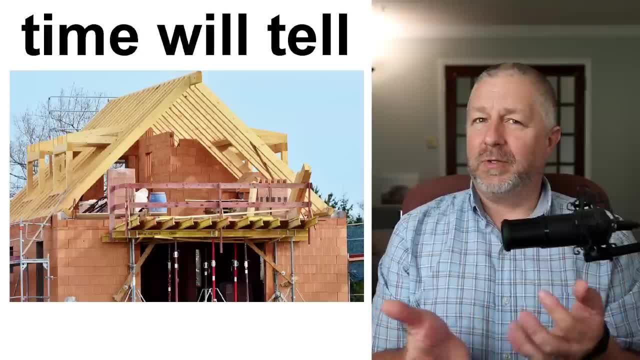 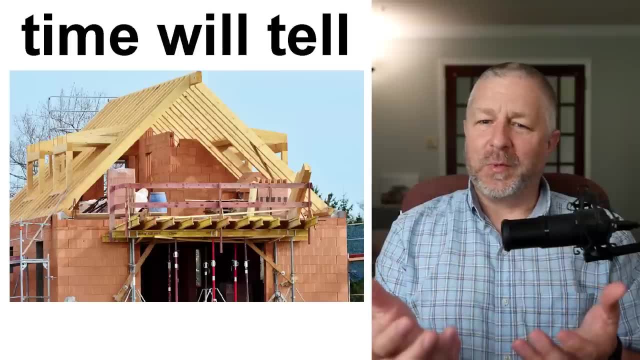 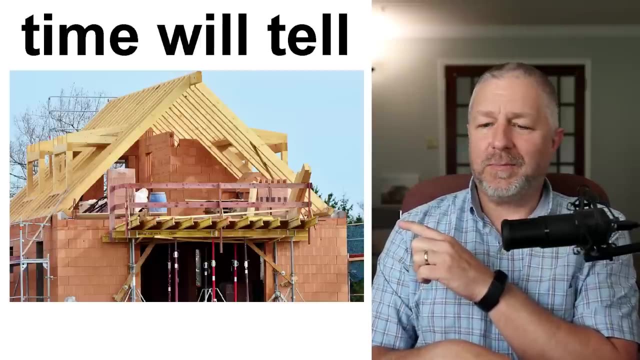 we use when we're not sure when something will be finished or we're not sure what the future will look like for someone. So here's a couple of examples: Maybe there's a house being built And they don't seem to be working on it very. 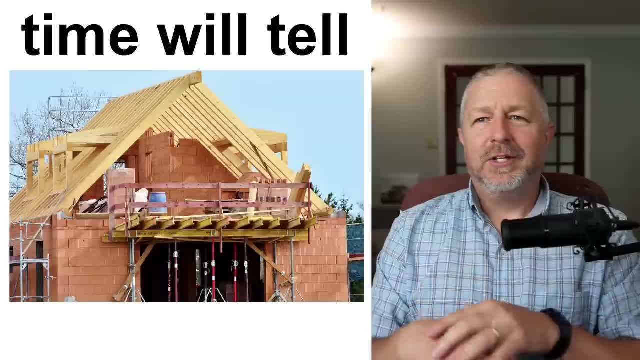 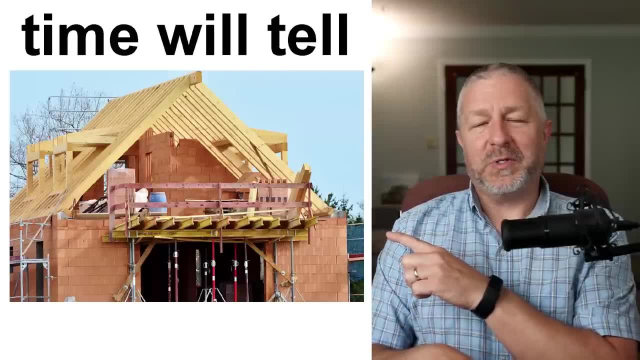 often You're not sure they're ever going to get done. So you could say, well, time will tell, Like if we wait long enough, we will find out if the house is going to be finished. And maybe you know someone who's in university and they're not. 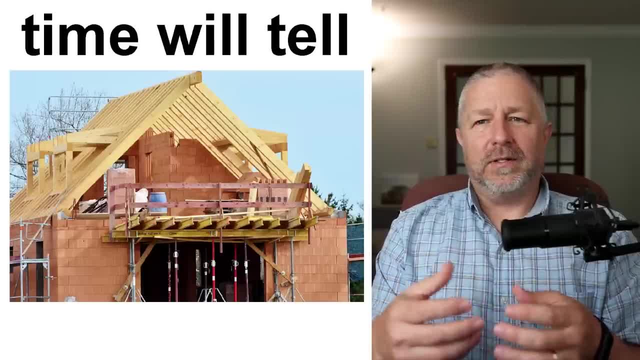 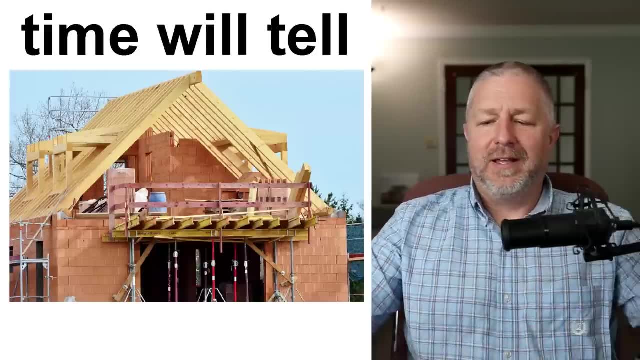 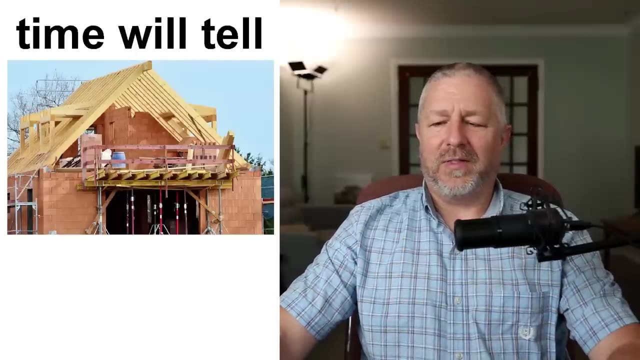 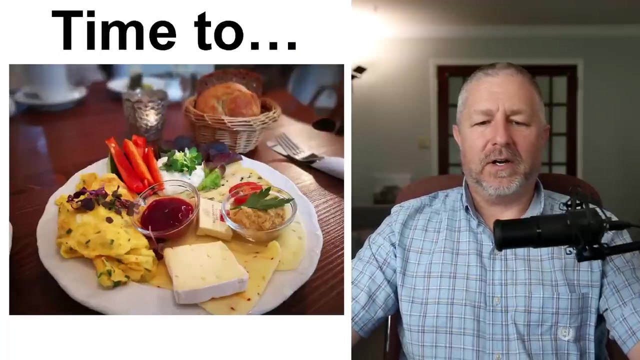 doing well And you might say: do you? someone might ask the question: do you think they'll graduate? And you can say: oh, time will tell. So basically you're saying, if you wait long enough, time will reveal the answer to the thing you are thinking about. Time will tell Time two. So we start a lot of. 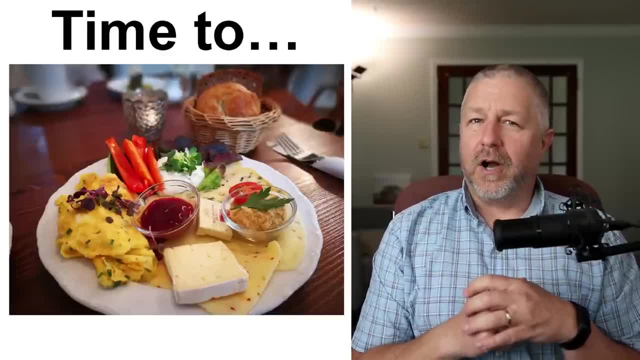 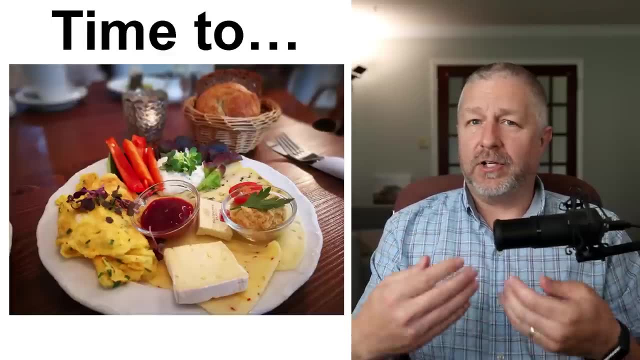 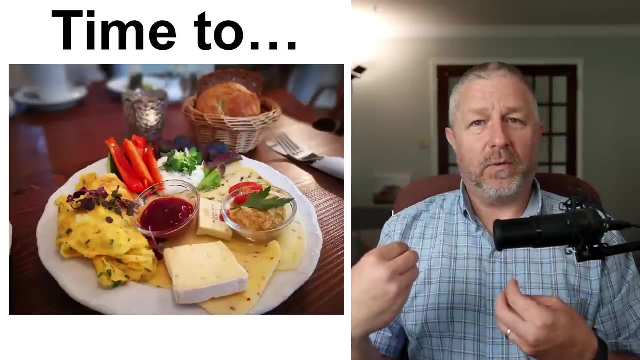 sentences with time Two. Um, probably a common one would be time to eat. So when I'm making supper, when supper is ready, after I'm done cooking the food in my house, I might say time to eat, Like I might yell time to eat. So my kids know that it's time to eat. I. 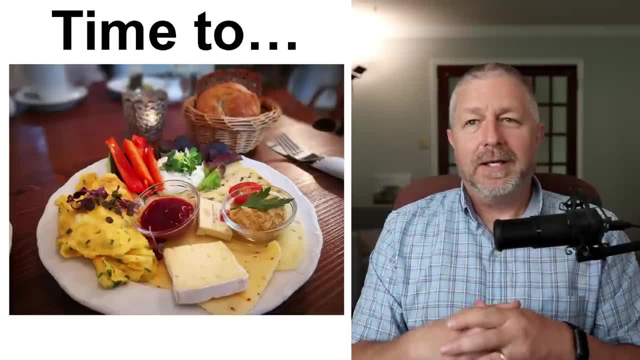 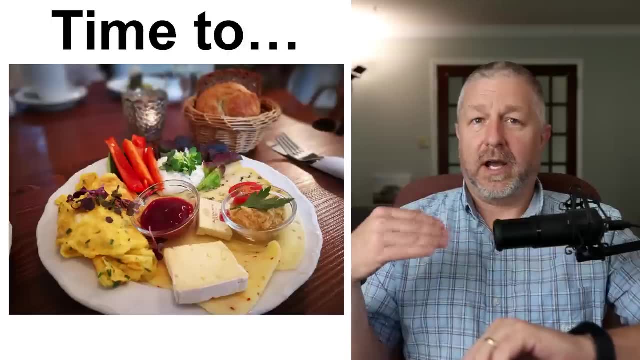 might text Jen and say time to eat, with a smiley face. We also say time to go, Like in the morning when we're getting ready, Um, when it's the time where we need to leave, I'll. I'll say time to go, Um. or my kids might say: is it time to go? 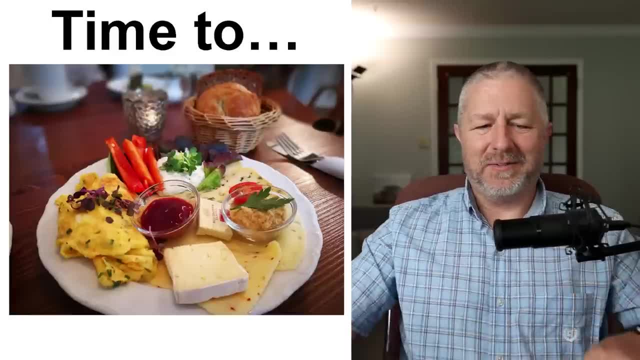 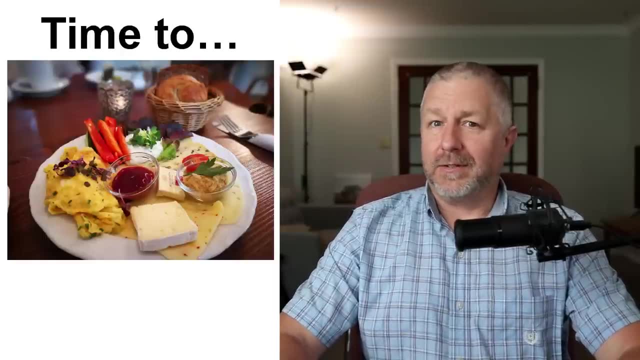 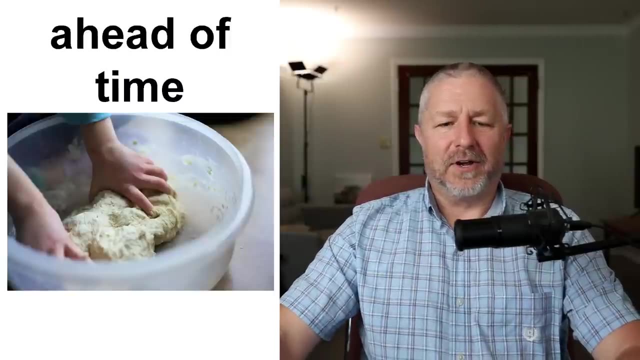 Is it time to eat? That's another common question in my house. So we do start a lot of sentences with this: Time to go, Time to eat, Um time to start the lesson. Uh, it's a. it's a fun way to start a sentence Ahead of time. So this person is 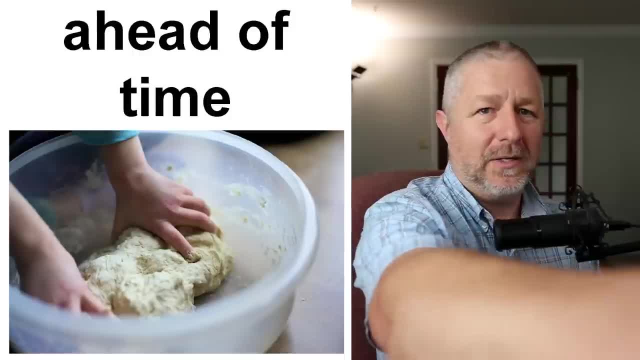 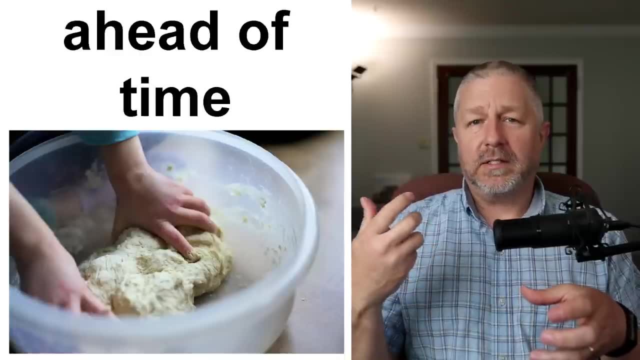 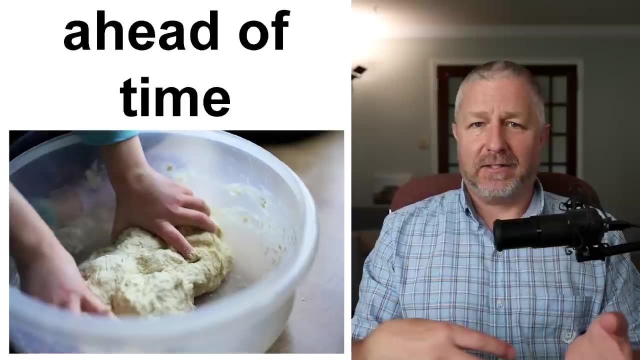 making dough. I'm going to assume they're making pizza dough. When you make pizza dough, you want to make it ahead of time. What that means is: if you want to eat pizza at night, you need to make the dough in the morning. You need to make it ahead of time. You can't make 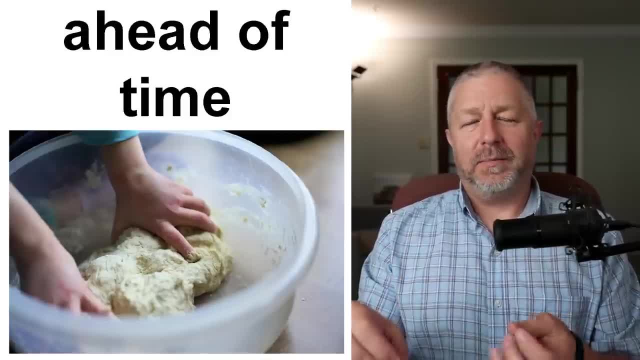 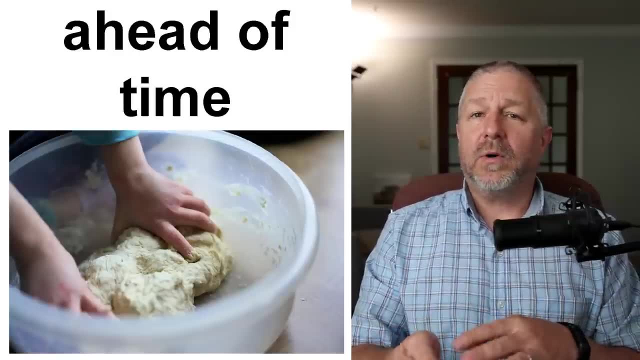 pizza dough when you want pizza, Because it has to rise and you have to knead it and it has to sit for a bit. It takes a few hours, So you make the dough ahead of time. Whenever you do something ahead of time, you do it before you actually. 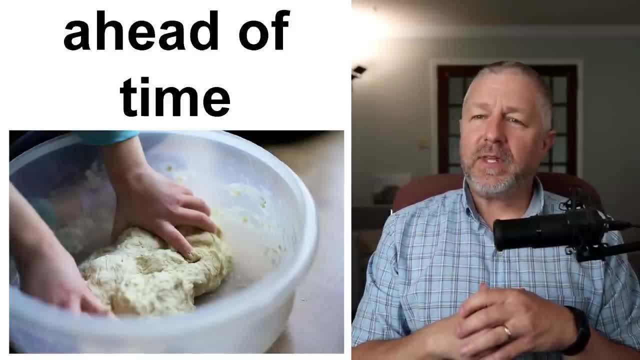 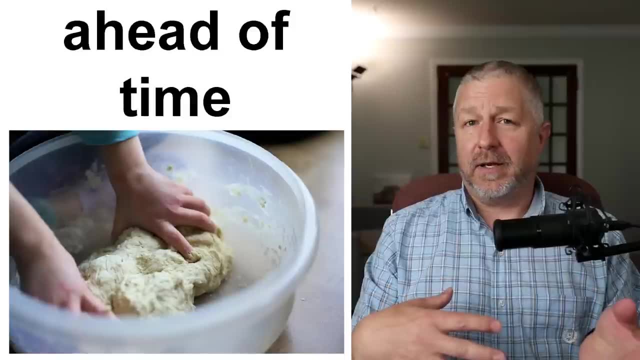 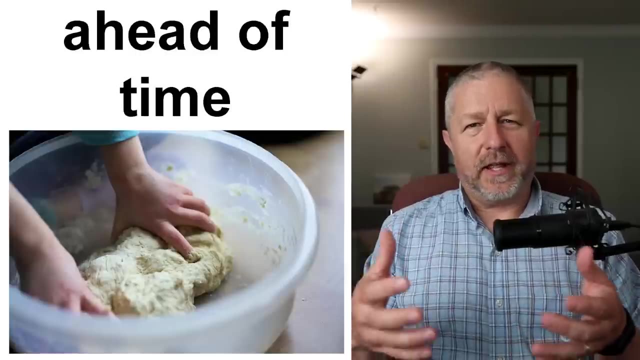 need it. So what's another good example? Um, if I was going to go for a bike ride, I would want to make sure. I would want to check the bike ahead of time to make sure the tires are pumped up. I wouldn't want to check over the tires and the. 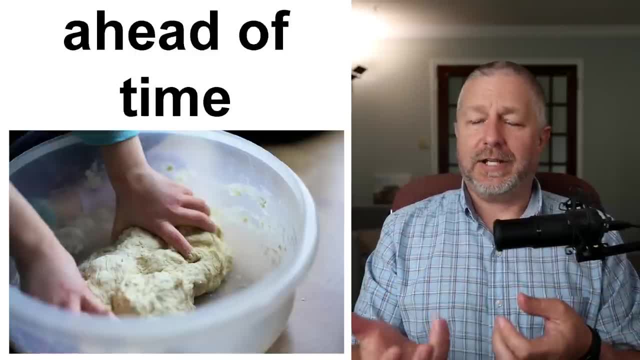 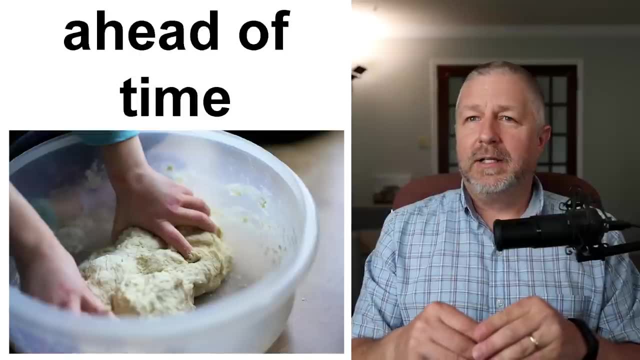 bike the minute I want to ride. I want to do that ahead of time. Um, let me see what's another good example. I'm trying to think of another good example. Cooking is a great example, right? Um, if you have a lot of people. 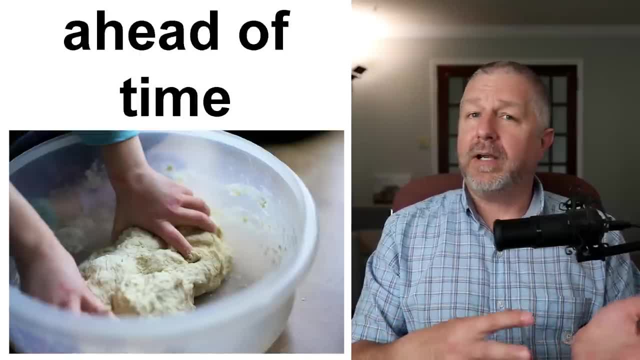 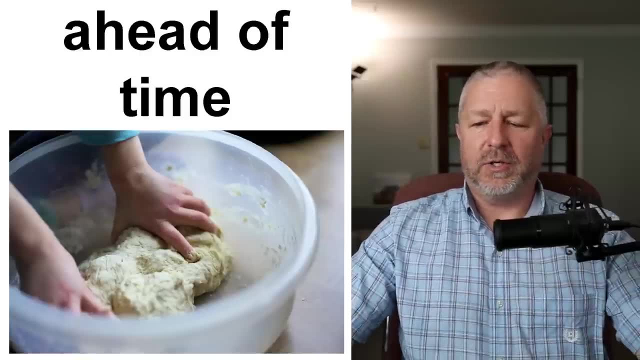 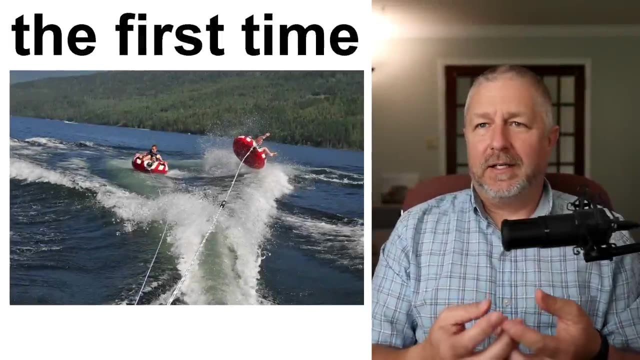 coming over and you're making a big meal, you might want to prepare some of the ingredients ahead of time. You might want to chop up the vegetables and have everything in the fridge ready to go. You want it ready ahead of time, The first time. So when you talk about doing things, if it's 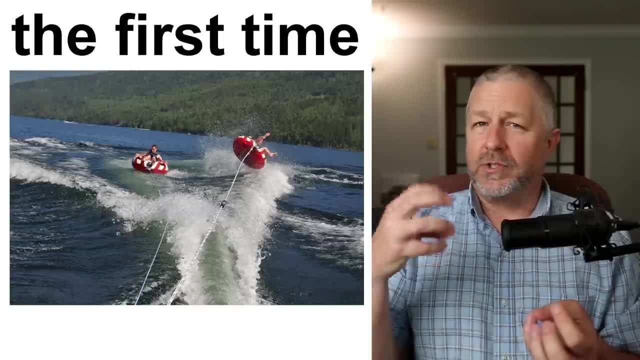 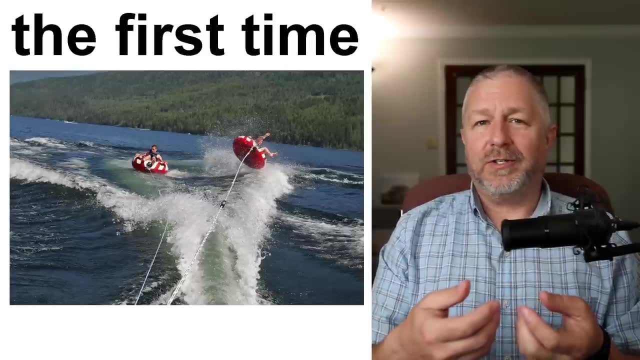 something you've never done it before, then when you start doing it, that's the first time. So the first time I rode a bike, I fell off. The first time I tried to skate on a ice, I fell Um. the first time I drove a car, I was really. 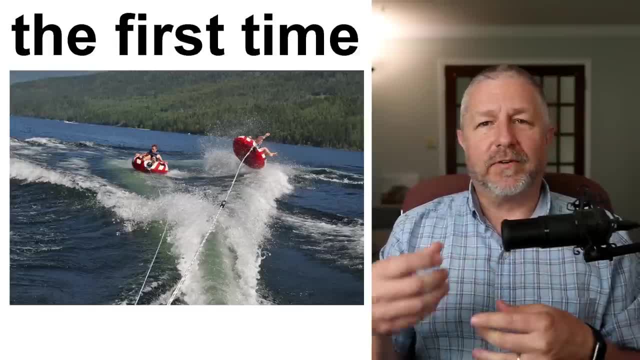 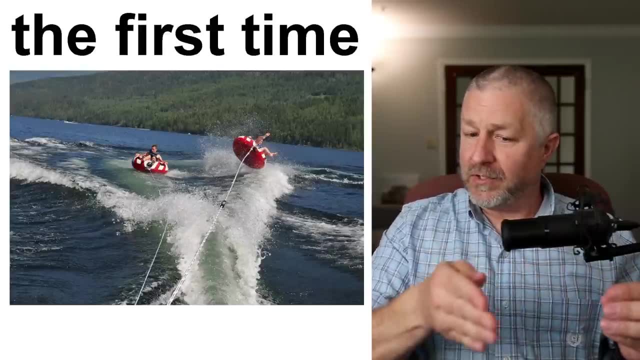 really scared. I didn't like driving when I was 16. So the first time. So whenever you talk about something that you that you've never done and then you start doing it, that there's always the first time. okay, Um, the first time I climbed a. 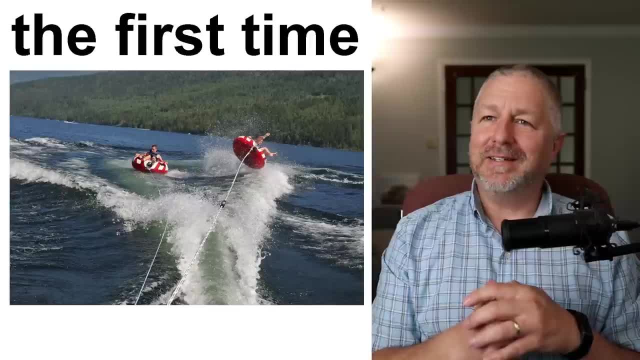 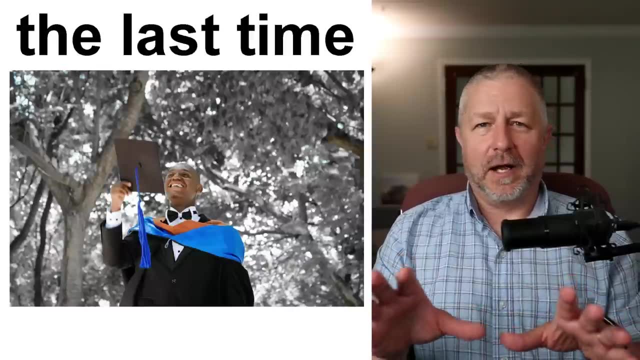 tree. I fell. I fell out. I remember that as a really little kid, the first time I climbed a tree, I think it was the first time. Um, we also have the last time, And this kind of has a couple of meanings. So one would be this: Uh, this person is. 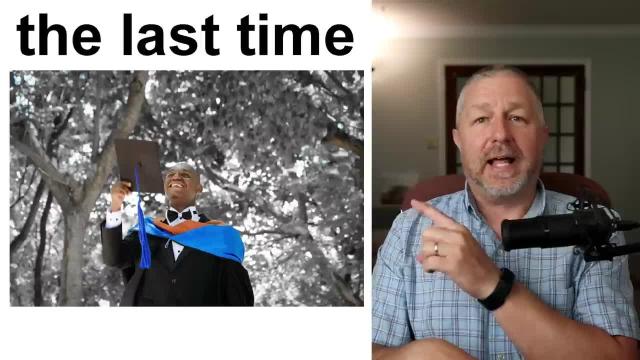 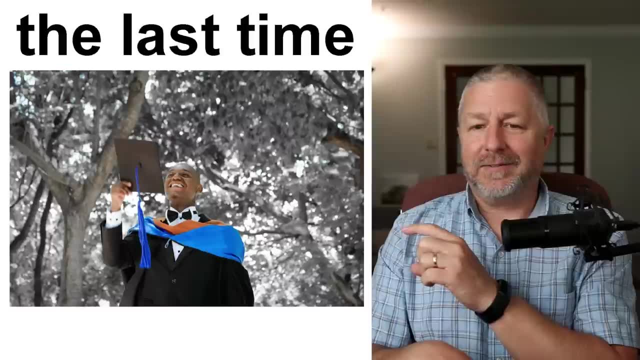 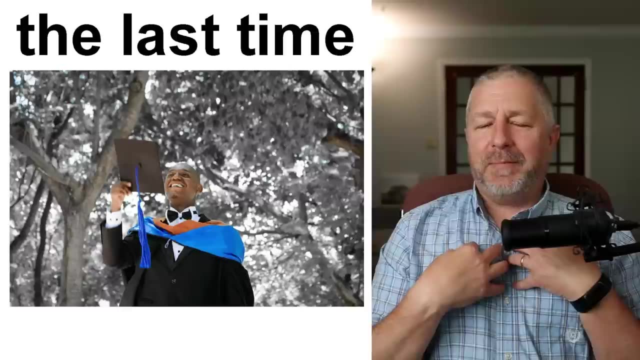 obviously graduating. So, um, this is the last time that they'll be at this school, This is the last time that they have to write an essay. So the the time it's when you don't have to do anything anymore. So I was happy, because when I 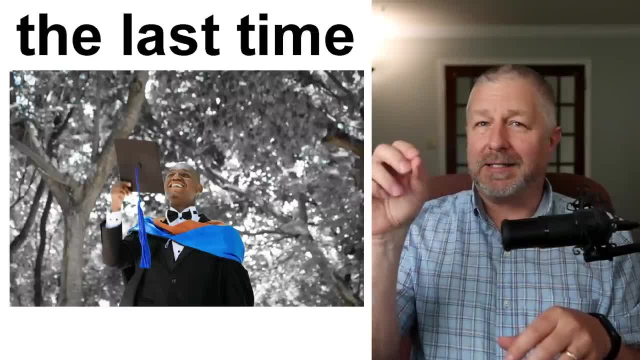 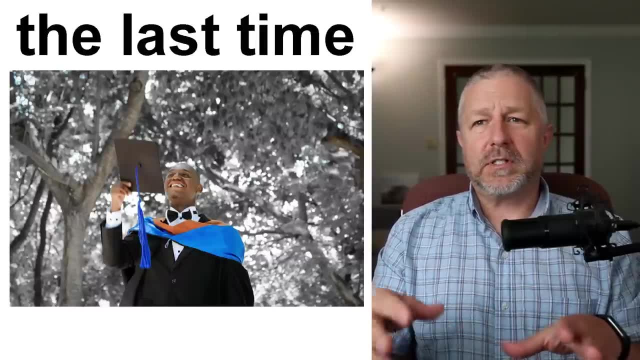 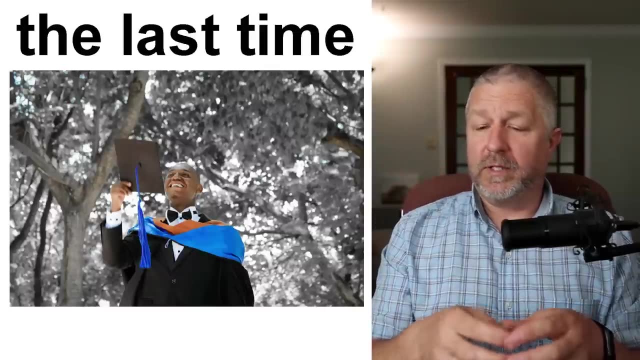 finished university. um, when I wrote my last exam, it was the last time I would have to write a test And although I did do tests after that, We also use this to talk about the most recent time that we did something. So the last time I drove my van was about an hour and a half ago. I 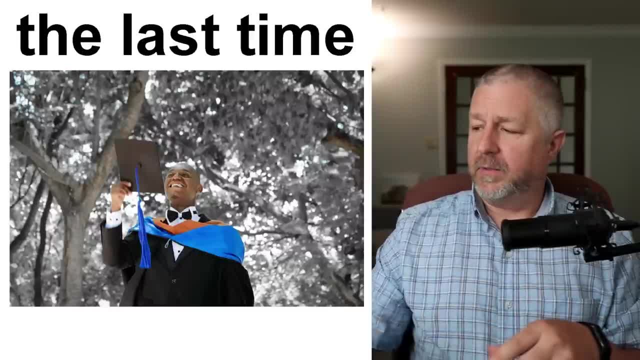 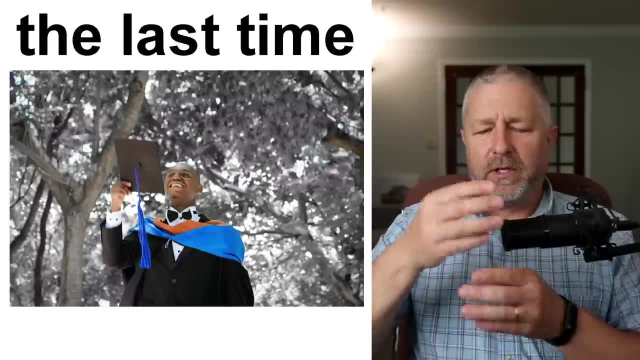 brought one of my kids to work. The last time I had a sip of water was about three minutes ago, So I'm going to have another sip now. So it can mean you know you're doing something in life and then that point where you stop doing it, that's. 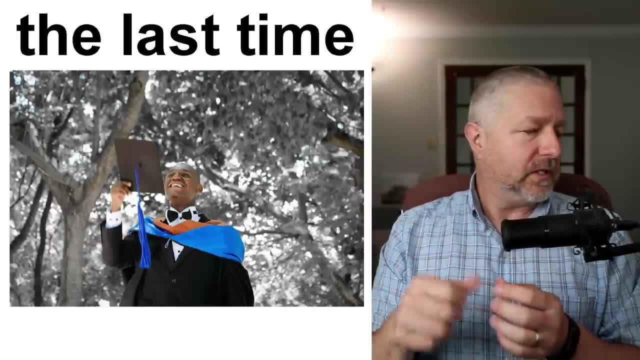 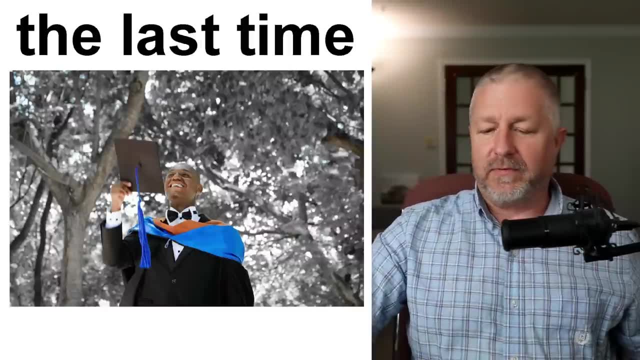 what it means. Um, but I can also refer to the most recent time. You know, the last time I held up my phone was five minutes ago. And here's my phone again: It's broken. I'm sad. So couple different meanings there Next time. So 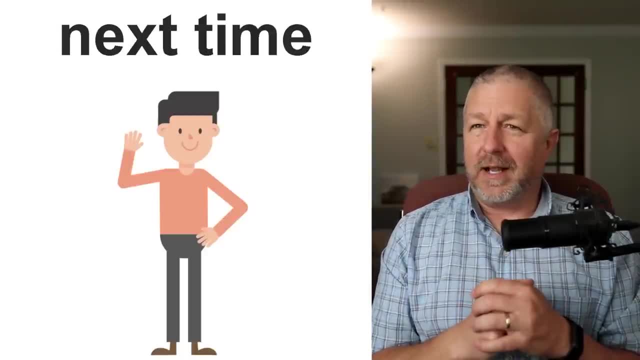 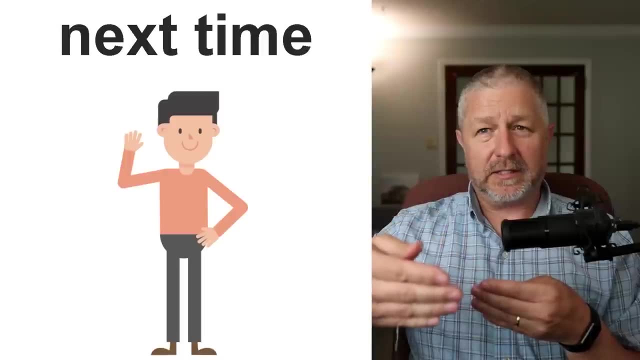 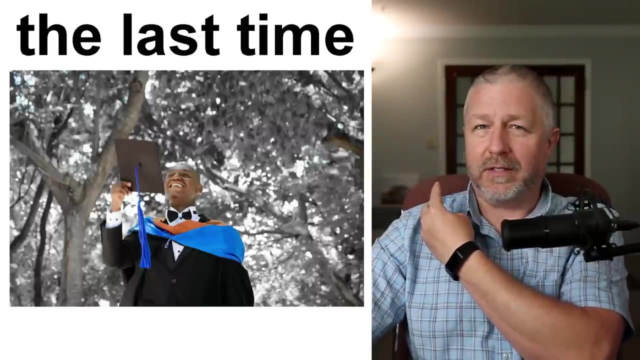 next time I'm going to teach a lesson, I think about gigantic things. So I'm referring to. there's a series of English lessons, and I'm talking about next time As opposed to last time. Okay, Uh, last time I talked about tiny things, right? Was that last week? This time I'm. 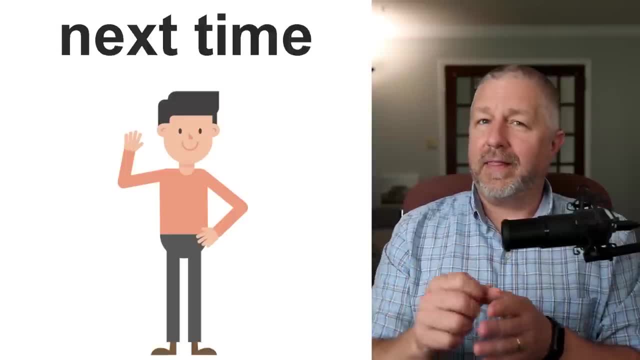 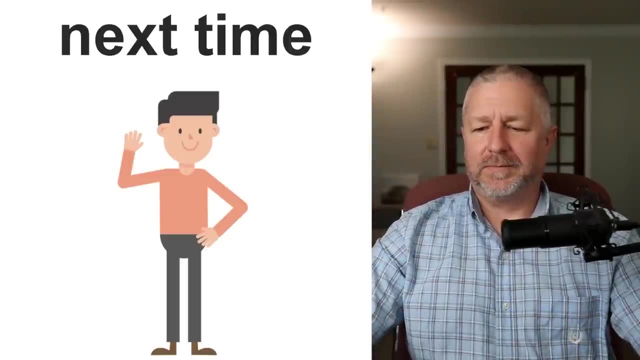 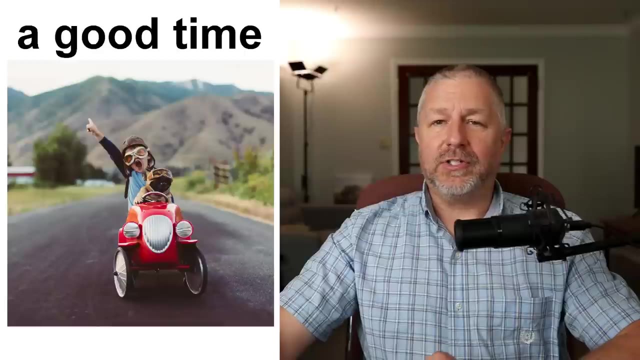 talking about um time phrases, and next time I think I might do a lesson on gigantic things. We'll see That lesson's half done. I'm not sure I'm going to do it. A good time: When you are enjoying something, you are having a good time. I hope that. 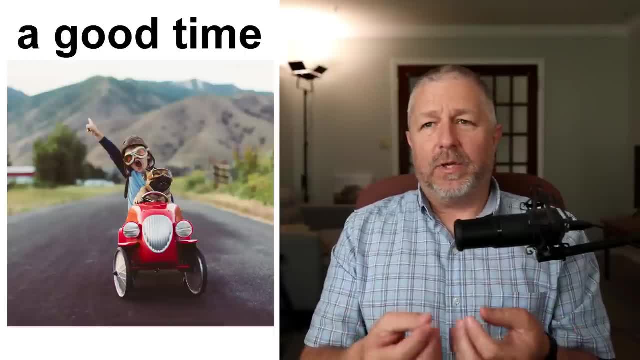 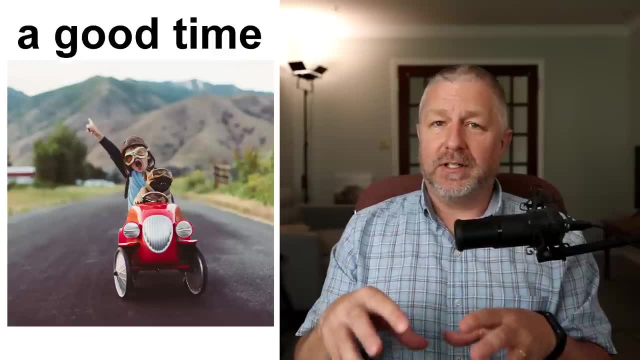 when you watch these English lessons, you have a good time. When you have a good time, you're happy. You're enjoying the thing that you are doing. I have a good time when I'm teaching these lessons. Um, I have a good time when Jen and I go see a movie. It's a good. 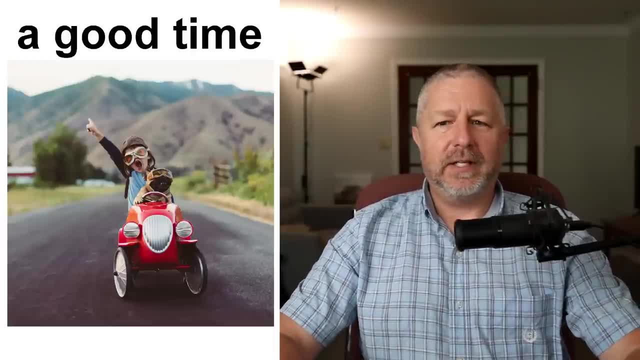 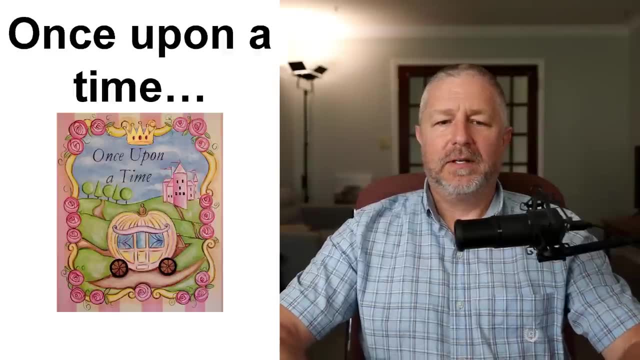 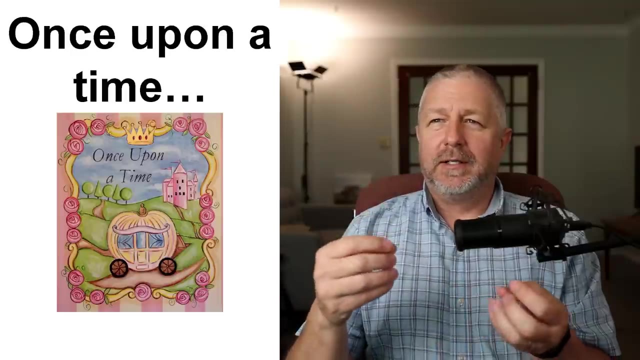 time We have a good time together. So a very simple phrase, but I hope that most of you are having a good time right now, Once upon a time. So this is how a lot of fairy tales start. Fairy tales are like old stories about you. 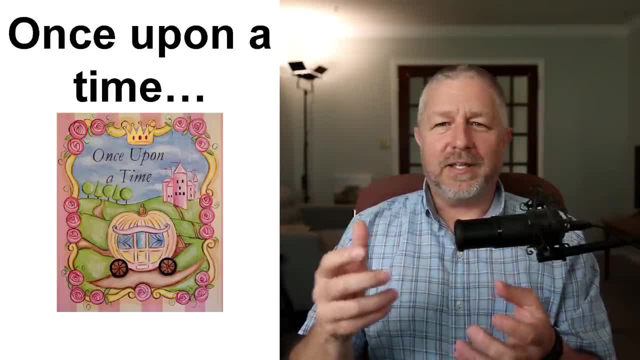 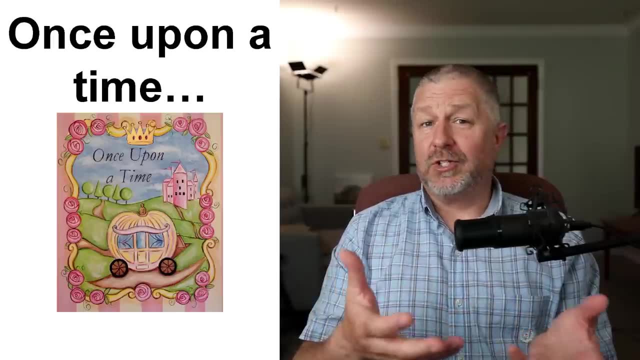 know wizards and knights and those kinds of things, And I'm sure a lot of you are familiar with fair maidens, So they often start with. once upon a time There's a TV show, I think, that has this as a title, Um, but you might have a story where it's 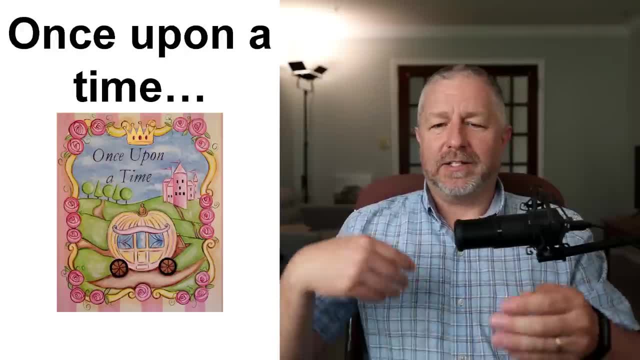 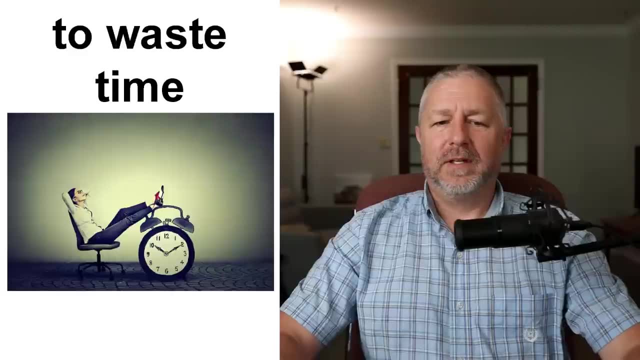 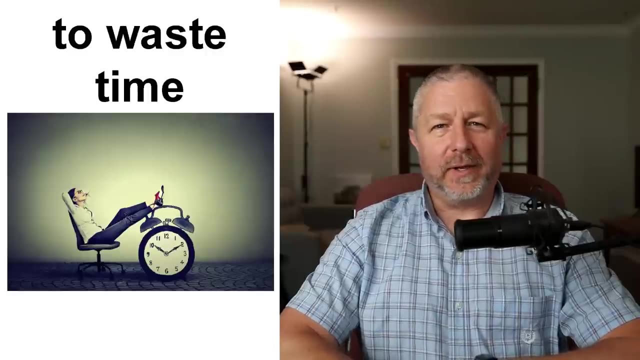 like once upon a time there was a man who lived on a farm And it tells the story and that's how it is introduced. A very common way to introduce that To waste time. So I don't like it when my kids waste time. I actually don't like it when 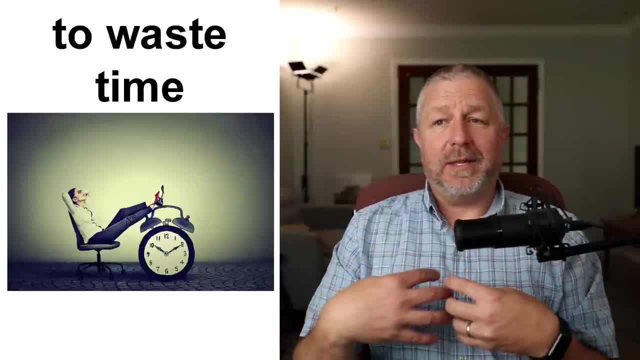 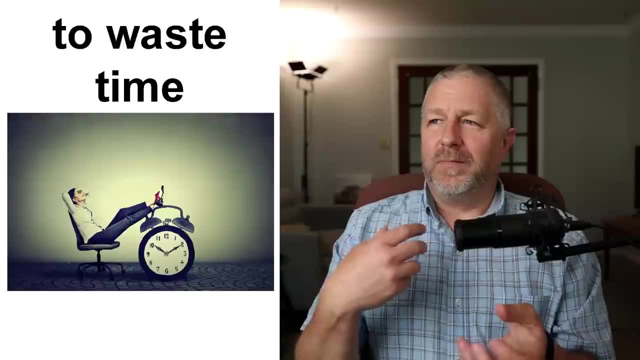 anyone wastes time. I don't like it when my kids waste time. I don't like it when my kids waste time Sometimes at work. I'm in a meeting and someone will talk forever and I don't like it because they're wasting time. when they do that, I'm they're. 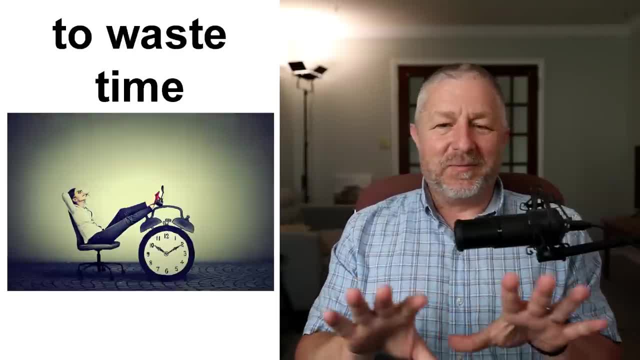 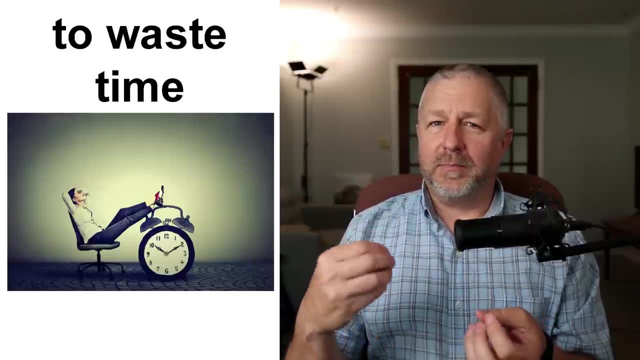 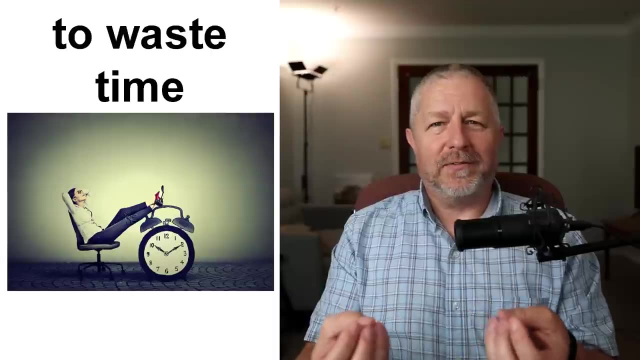 not contributing to the meeting, Sorry. Hopefully none of my colleagues are watching. So when you waste time, you are not working hard, You are not being productive, You are not playing as a like a, you're not a good member of the team. So 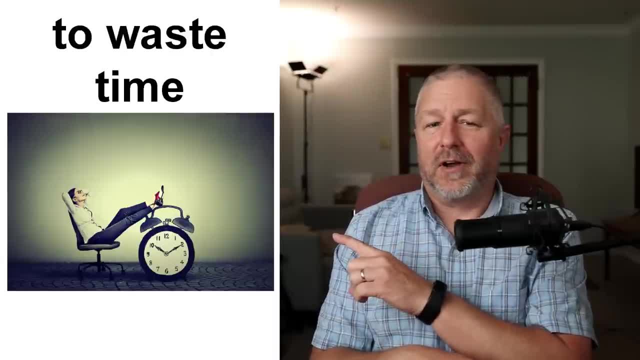 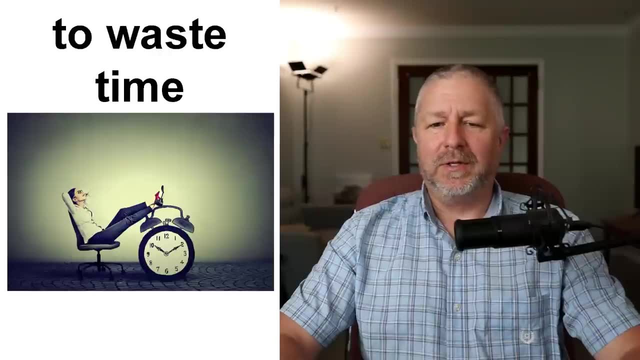 this person has decided to do this. So this person has decided to waste time. It's not good to waste time. I think in French it's. is it Gaspier? Is that the word, The verb Gaspier, In the chat? maybe someone can let me know. But to waste time It's. 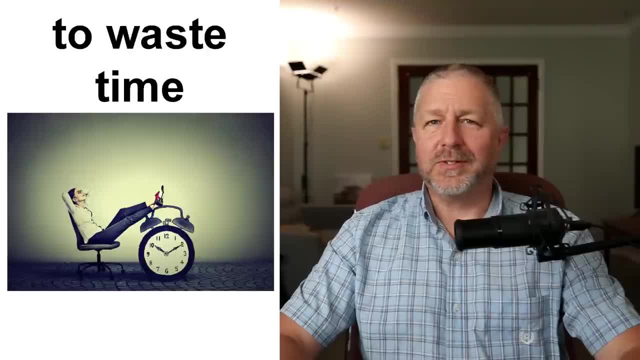 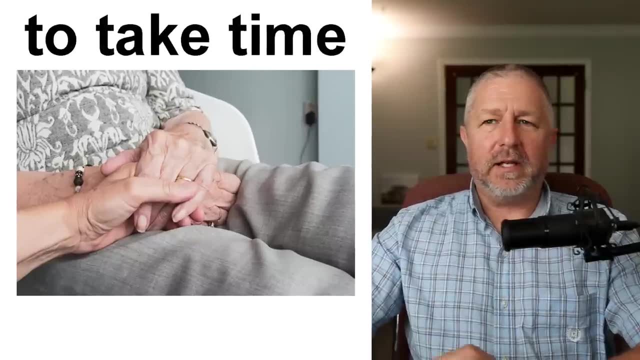 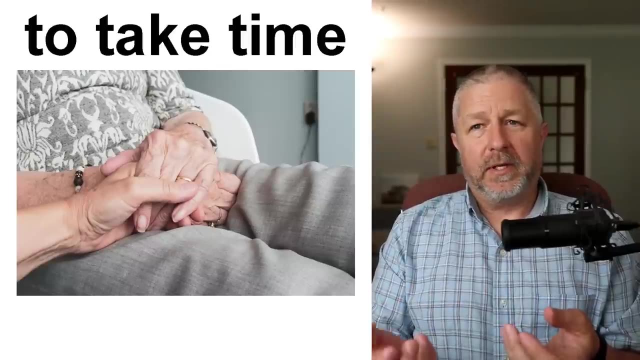 Gaspier or Gashy, I don't know. I should stop saying French words, because who knows what I'll say. To take time? Um, in English we talk about this when it's important to do something. So it's important to take time to visit older people. It's. 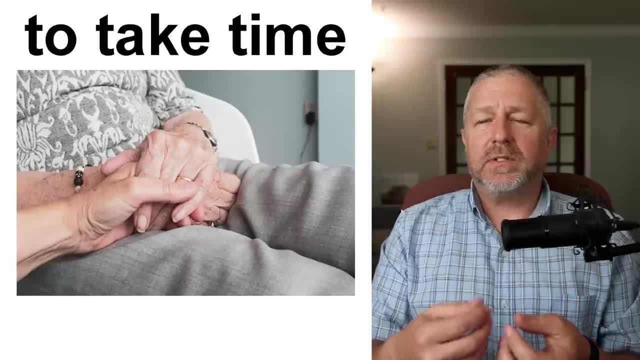 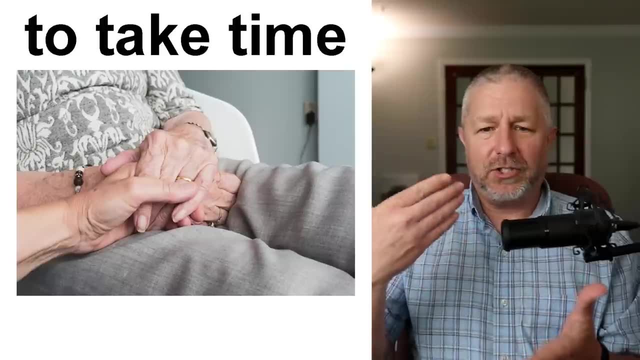 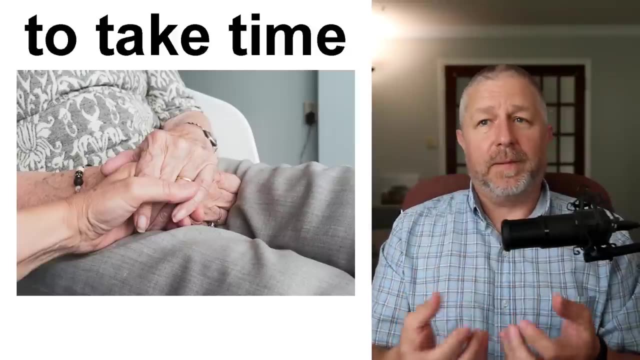 important to take time with friends. It's important to take time to do something properly. Okay, So when you take time, it means you intentionally decide to spend your time with some people. Okay, So you need to take time. Um, now I'm going to. 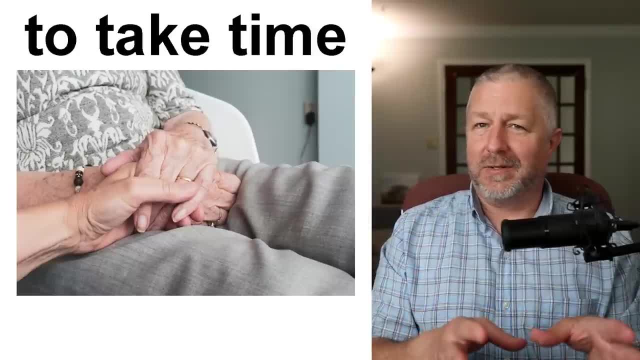 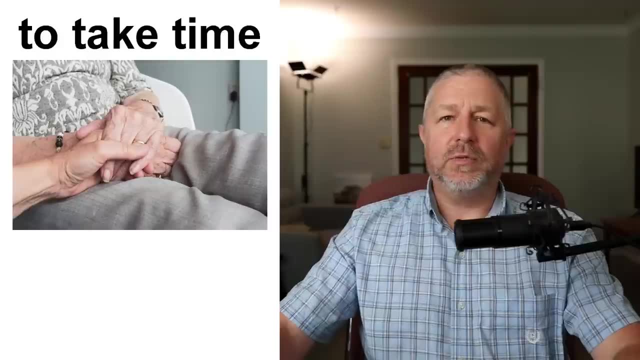 add a word here: When you take your time, it means to go slowly, But when you take time it means you intentionally decide. So I take time every week To visit my mom. I haven't actually visited my mom for a couple of weeks because I did just see her a few days ago. 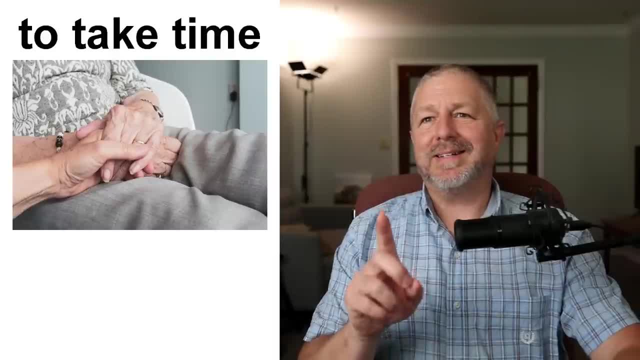 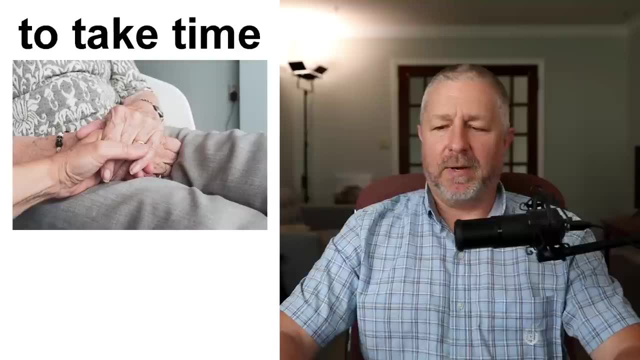 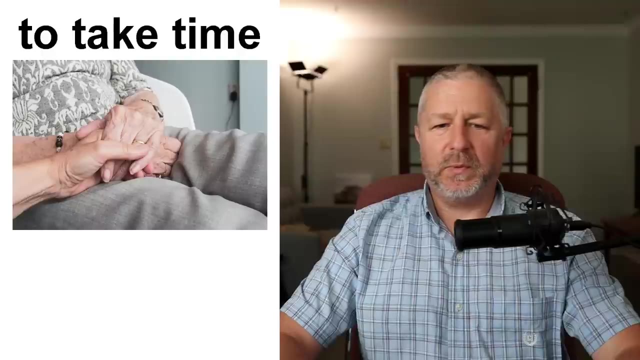 Not for my birthday, Just so you know, But I did just see my mom, Uh, a couple of days ago, Um. but usually I take time every week to visit my mom And Freddie Wolf says, yes, Gaspier, to have time. So simply put you: either have time or you. 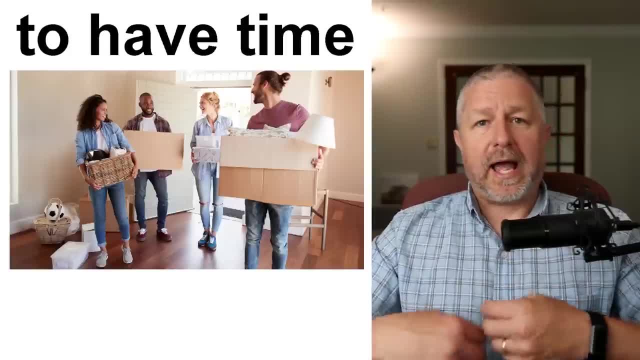 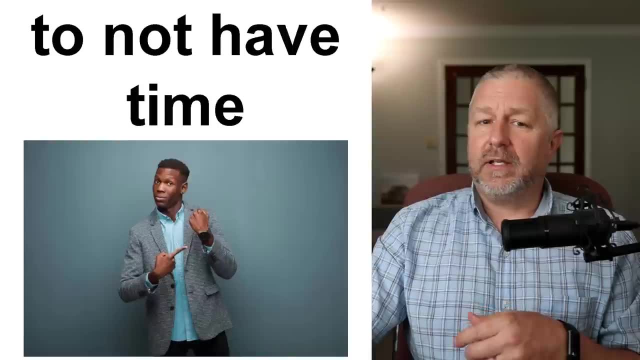 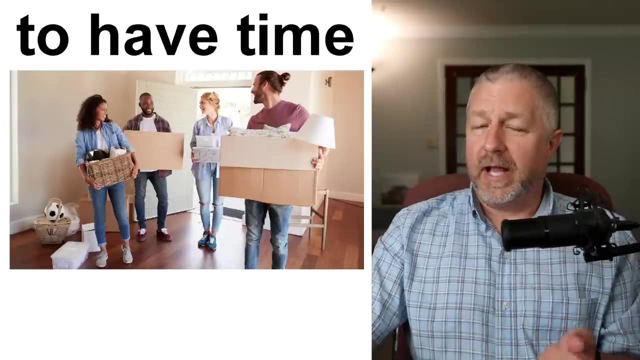 do not have time, I'm okay. So obviously you have time this morning to watch this lesson. I have time to teach this lesson. Maybe last week you did not have time And so you didn't come to the lesson. Maybe next week you will have time and you will be able to. 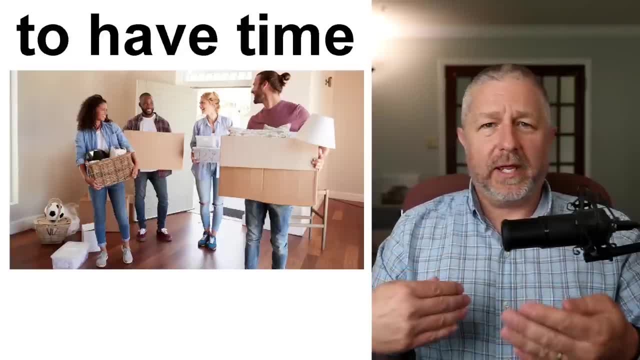 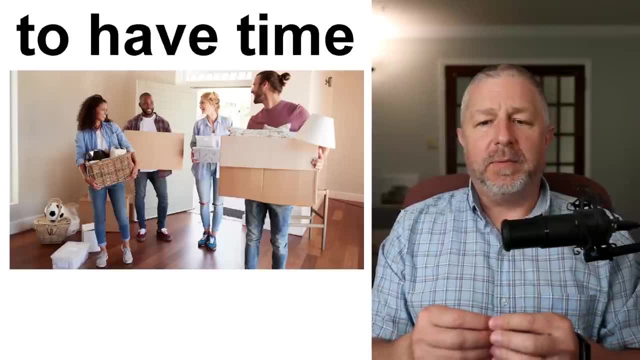 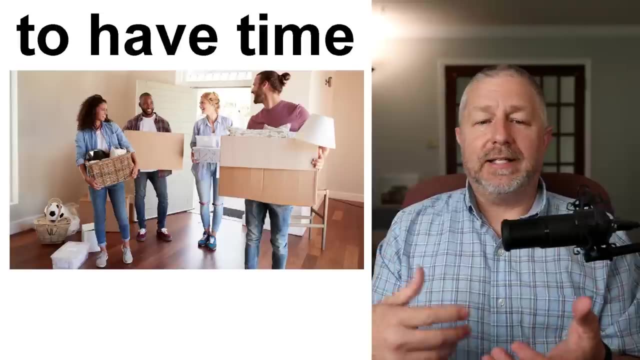 come to the lesson, So this is probably one of the more common ways to talk about whether you can or can't do something. Okay, Sometimes people will say: I didn't have time to eat breakfast. this morning I have some students who say: oh, I'm so hungry I didn't have time to eat. 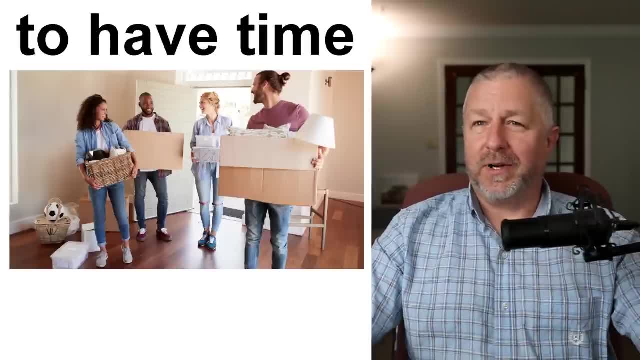 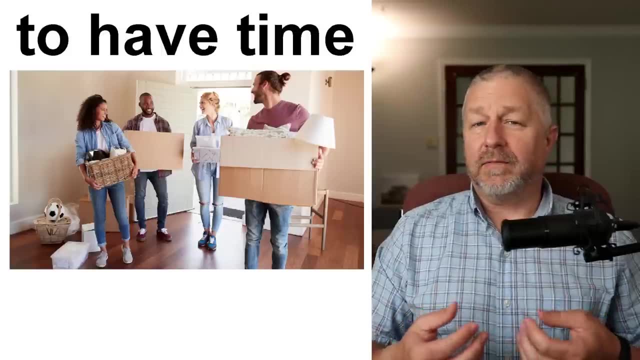 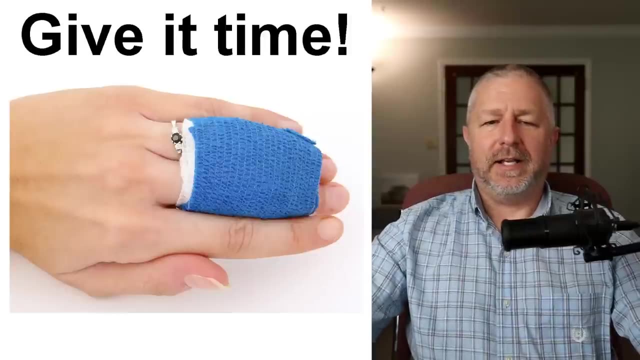 breakfast this morning. Um, it's not good to not eat breakfast. by the way, Sometimes students are like, oh, it's nice to have time to just sit and talk instead of learning new things. Sometimes students like to just have time to talk And give it. 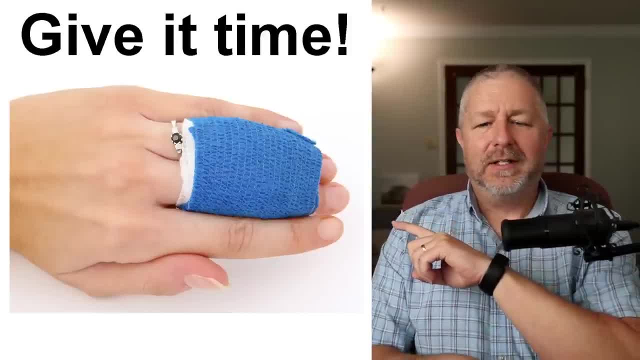 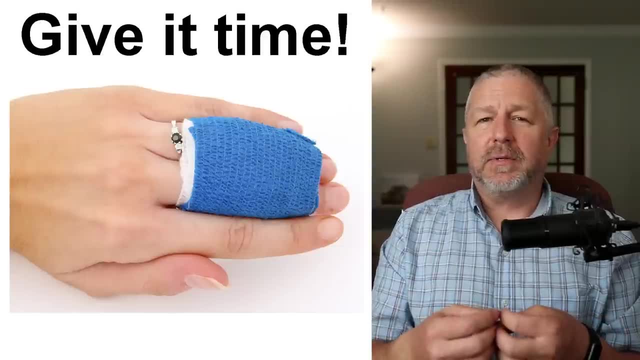 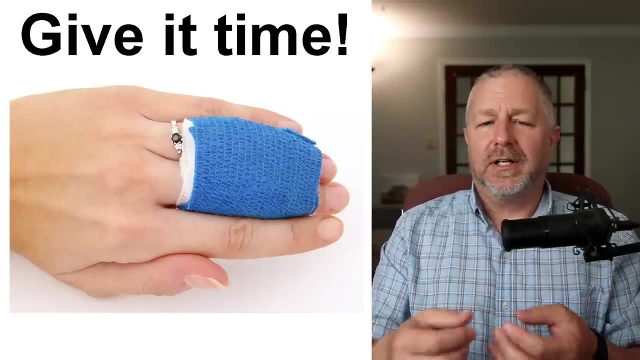 time. So this person obviously injured themselves, And one of the things that happens when you injure yourself is you get very, very frustrated, But sometimes you just need to give it time. You need to be patient. So basically, give it time means be patient. If you hurt yourself, you have to give. 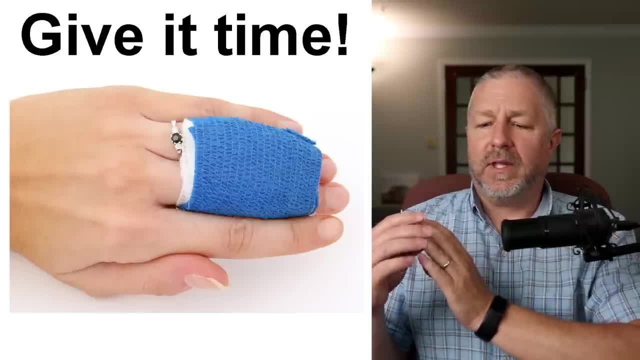 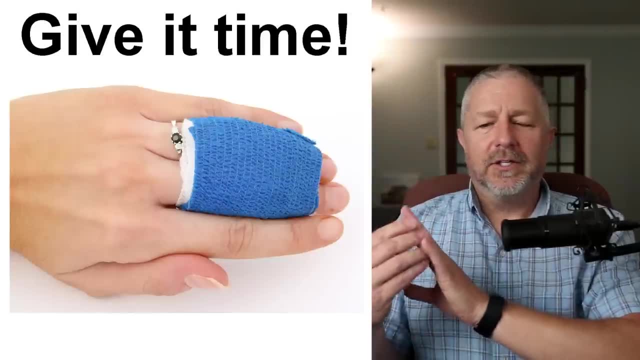 it time. It does not heal instantly. It won't heal by tomorrow, Okay, So you need to give it time. You need to just let your finger heal so eventually you can get back to doing the things that you want to do. You need to give it. 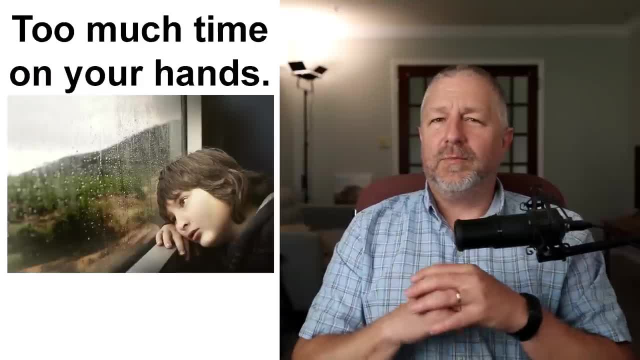 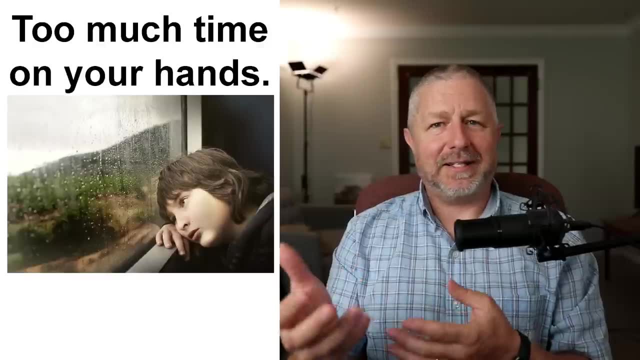 it time. Some of you might have too much time on your hands. I'm happy that you've come and that you are watching the lesson. I'm glad that you had time, but sometimes people have too much time on their hands or you might have too much time on. 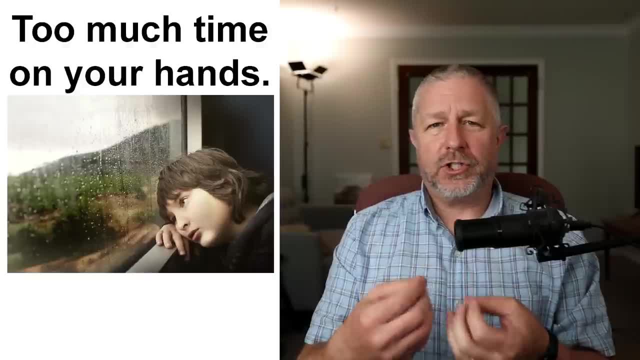 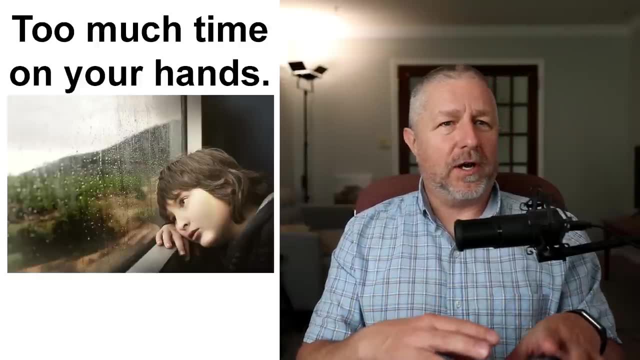 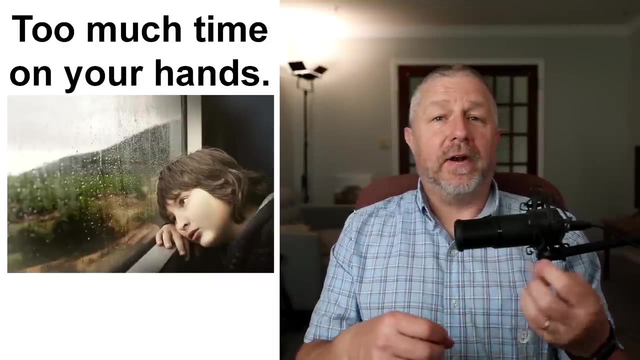 your hands. This is often true of children in the summer in Canada, because there's no school and they're too young to get a job and they don't know what to do every day. Maybe they don't have a hobby, Maybe they don't, Maybe their friends 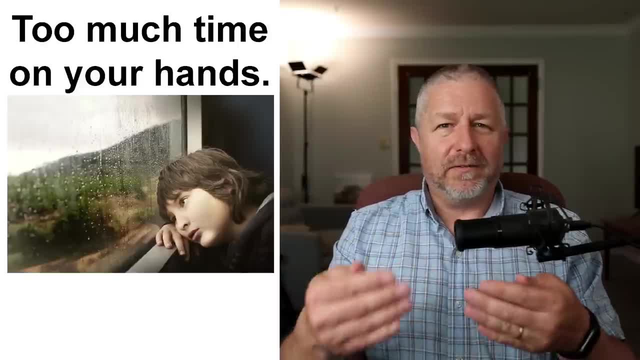 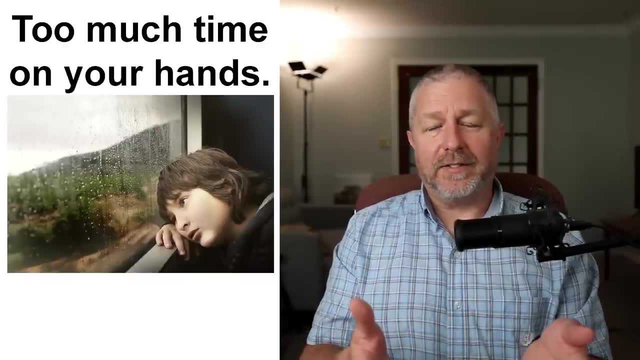 have all their friends, all have jobs. Maybe they're 14 or 15 and they just sit around and they're bored. We would then say that person has too much time on their hands. My mom now lives in an old, an old age home and she said she likes. 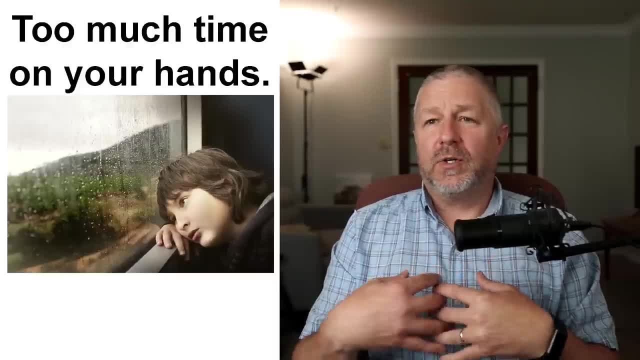 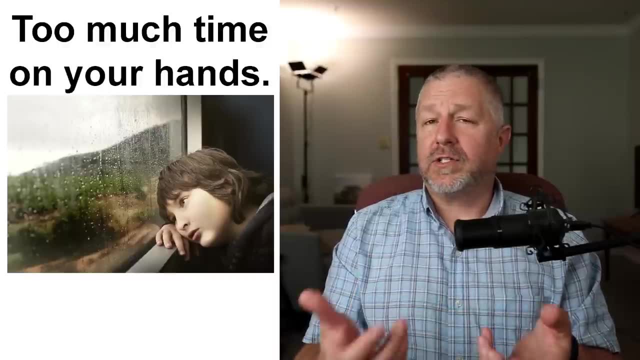 keeping busy because she has so much time on her hands. So she likes the fact that she can do different things throughout the day, because it's not nice to have too much time on your hands. It's nice to be busy doing things and learning.